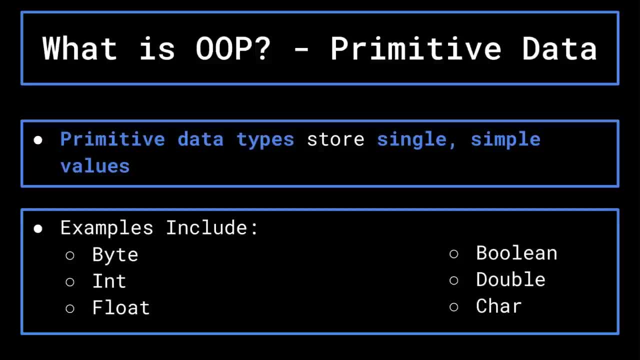 These primitive types only act to store a single piece of data of a certain kind, And for a while, when programming was still developing, this was just fine. Many programs being written at the time weren't complex enough to actually understand the data types They were. 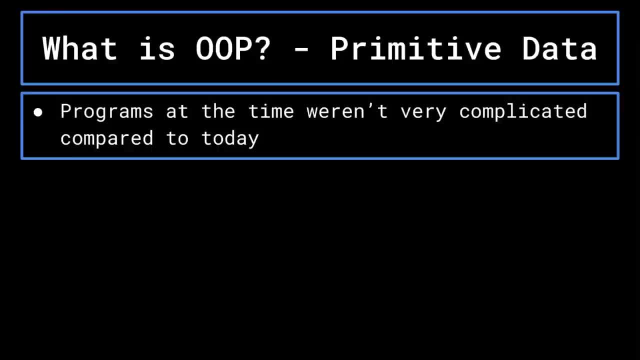 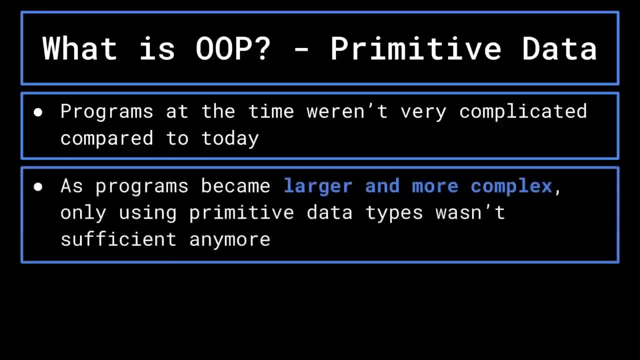 not designed to be used in any kind of programming, and they weren't designed to be used in any kind of complex by today's standards. Thus, programmers could get away with only using these primitive types. However, as programs became larger and more complex, primitive data types weren't 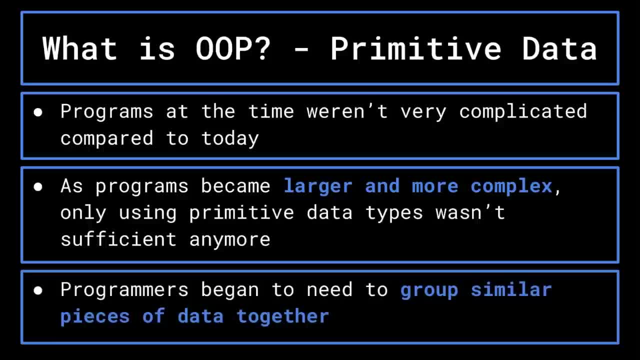 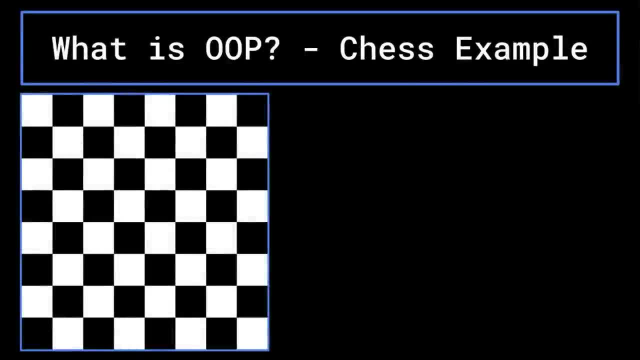 really cutting it anymore. Programmers began to want to group variables of similar type together. Why would this be useful? Well, to serve as an example. let's imagine you are trying to program a chess game. When programming a knight into the game, there are plenty of 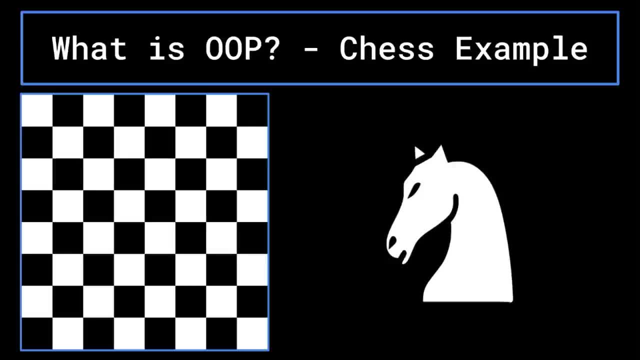 variables that you will need in order for the piece to work how it should. For example, you would need a position variable to keep track of where the knight is. Additionally, you would need a boolean to represent whether the piece has been captured or not, because 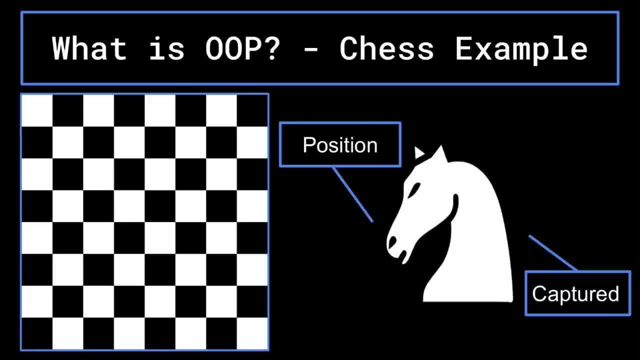 if it has, you would not want it to show up, nor should you be able to move with it. You may also need a variable to represent which color the knight is, so that the game can treat it correctly. These are just a few of the variables that you will need to keep track of where the knight 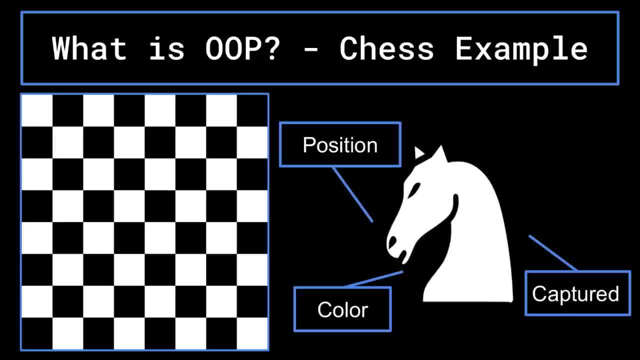 is, and you will need one of each of these variables for each piece on the board, each of which would contain different data. Clearly, it would be easiest if you could group all of the variables related to, say, one of your knights together so that you may deal with. 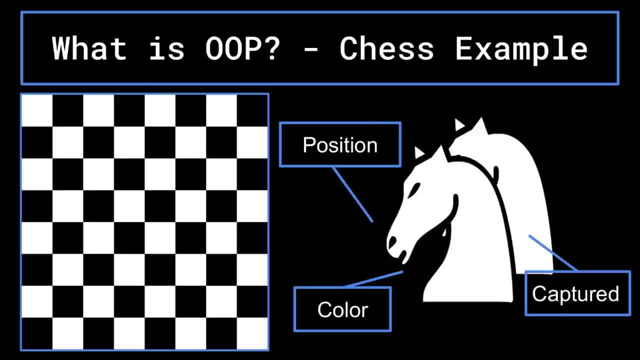 them as one entity. Additionally, you may want to group your two knights together, as they behave similarly. You then may want to group the pieces of each side together, as they would be treated differently in reference to each other. In essence, grouping related variables together is almost necessary when it comes to complex. 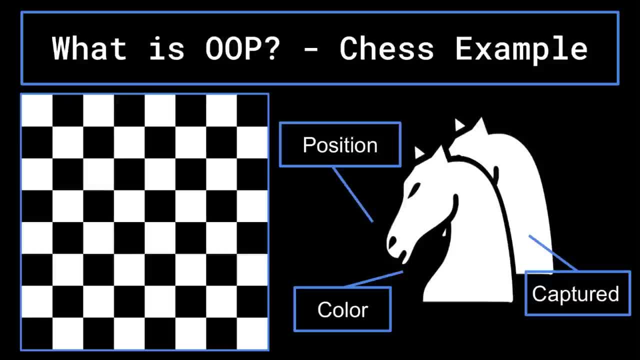 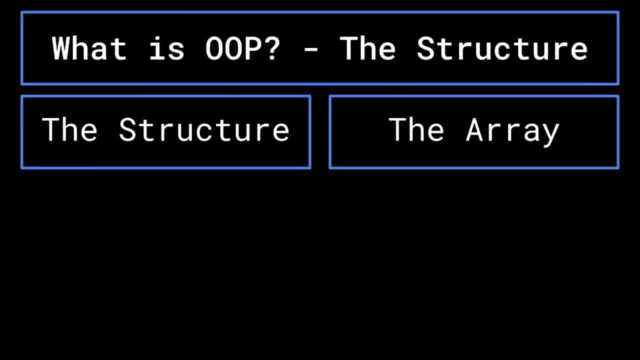 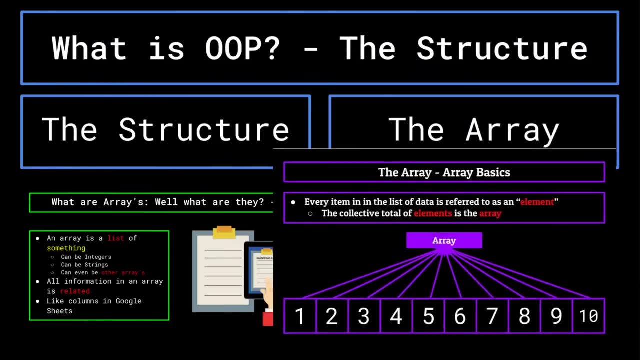 programs. This is where the struct or structure came in. In C, the structure is similar to an array. If you don't know what an array is, I'd suggest you check out either our Introduction to Programming course for an overview or our Data Structures series for a more in-depth. 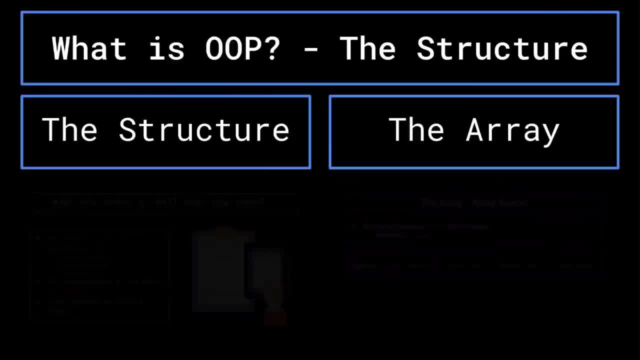 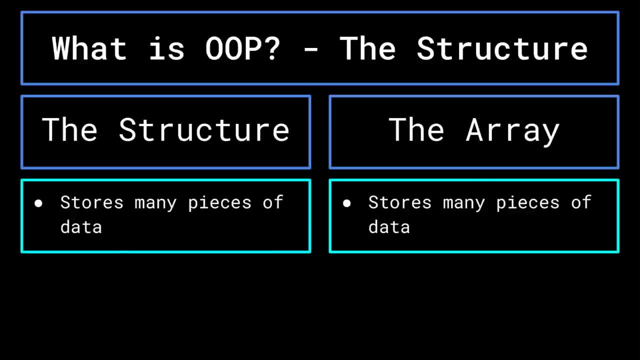 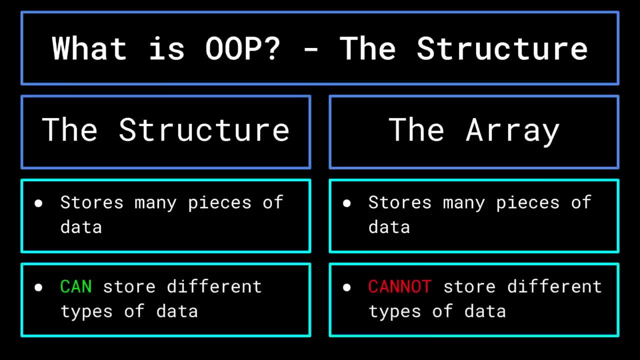 look at both arrays and structures. Both arrays and structures allow the programmer to store several pieces of data together. However, structures vary from arrays in that structures allow the programmer to store data of different types together, For instance, whereas an array would allow you to store. 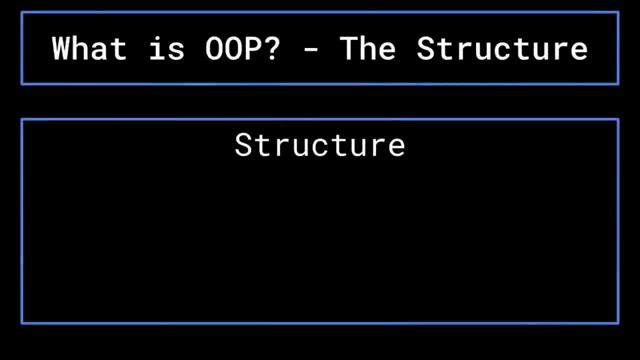 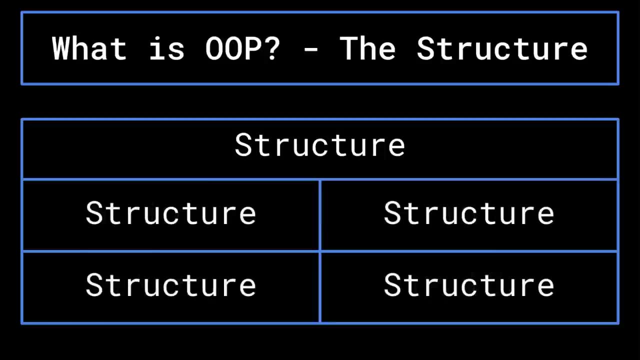 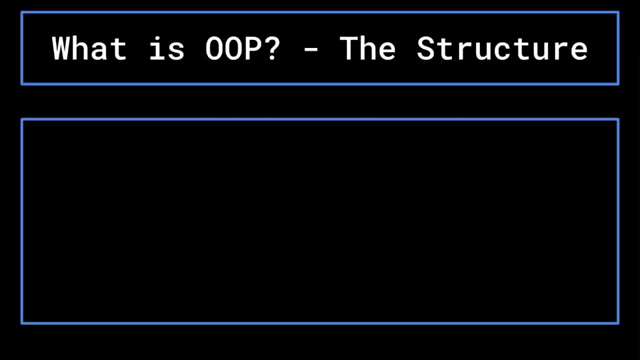 only ints or only strings? using a structure, you could store ints and strings together along with other data types. A structure can even store other structures, store other structures within it. A structure can be very useful in the earlier chess example because you could store all of the useful pieces of data related to the night in one structure. 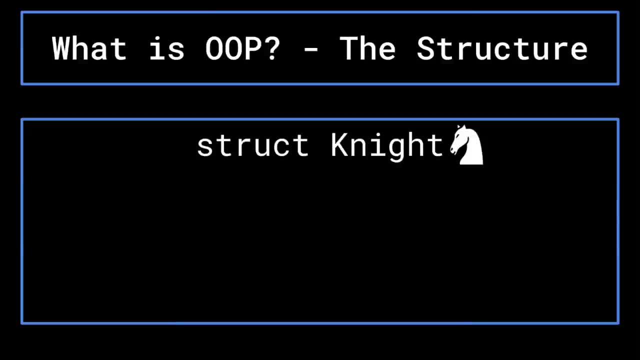 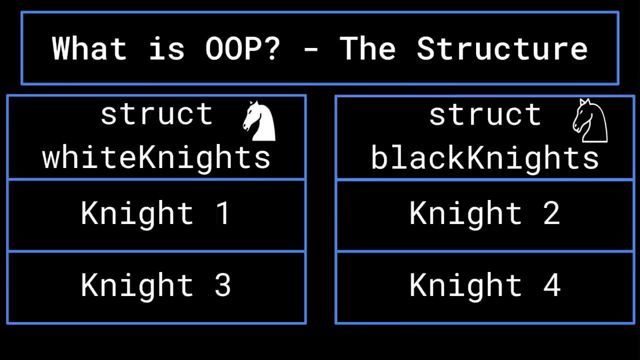 that represents that night. you could then store your night structures together in one structure that represents all of the nights, and so on. The structure allowed such grouping to take place beyond what arrays were capable of. The structure is, in many ways, the precursor to the object. 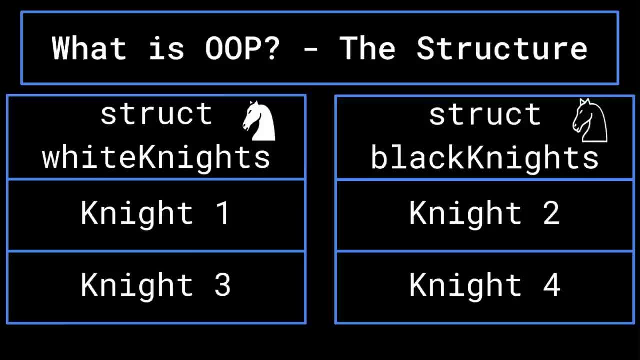 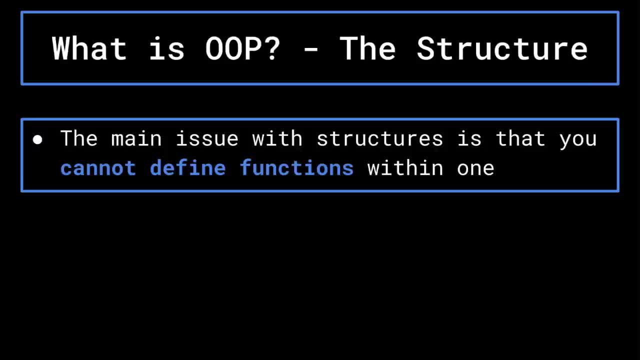 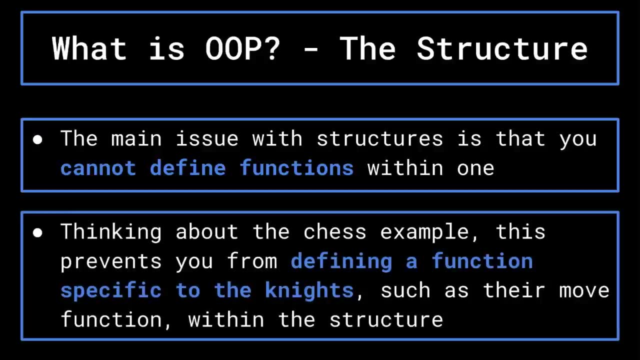 which, of course, object oriented programming is oriented around. the main issue with using a structure in this way, And an issue that objects would come to remedy, was that you could not define functions within a structure. you could only reference them When object oriented programming 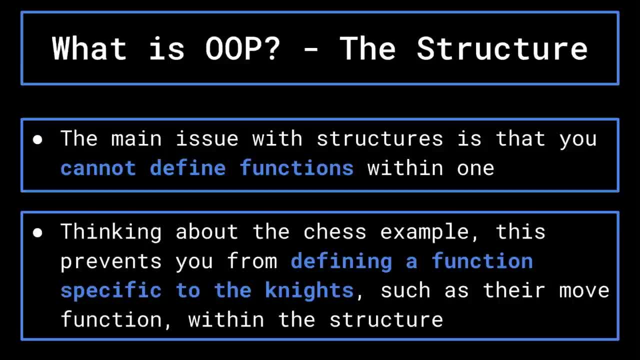 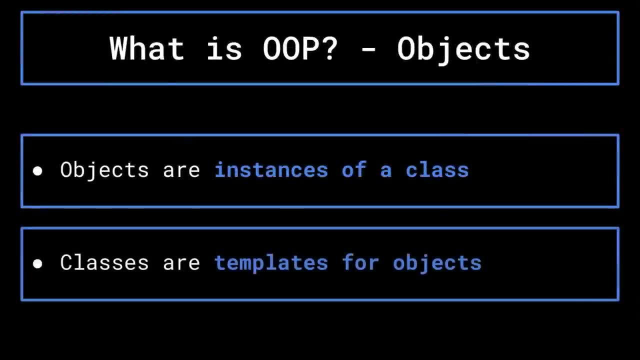 came along, objects allowed you to store data of all kinds together And, additionally, to find and store functions. Now, before we go much further, I should get into exactly what object oriented objects are. Objects are instances of a class, And a class is basically a template for an object. 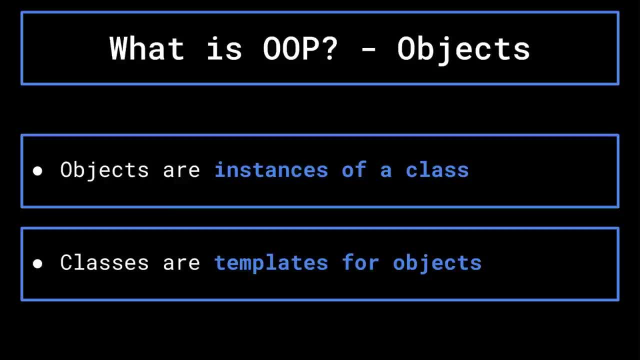 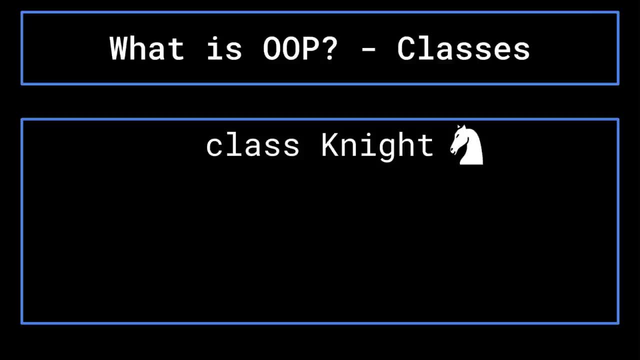 This may seem like a circular way of looking at these concepts, But allow me to explain. Let's say I define a night class. In this class, I would define and store data that is common of all nights. This would be mainly the way that nights are able to move. Thus, in this class, I would 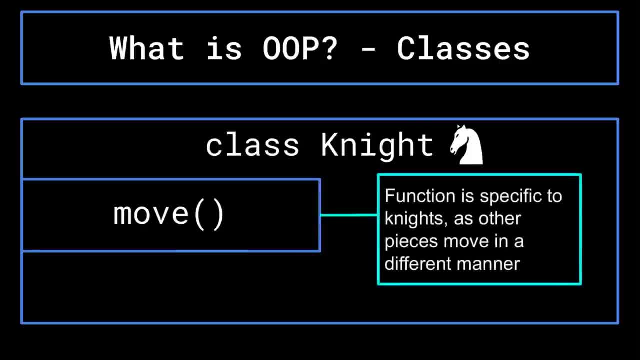 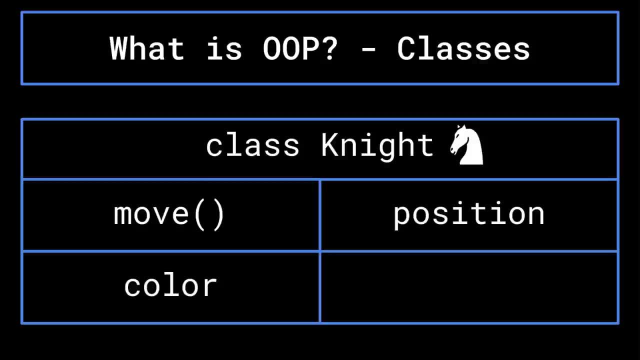 define a function that uses the nice current position To return squares that the night can move to. I may also define a position variable as well as a color variable, But I would not initialize them When it comes to specific things, such as variables that each object under the class, in this case each night, would have. 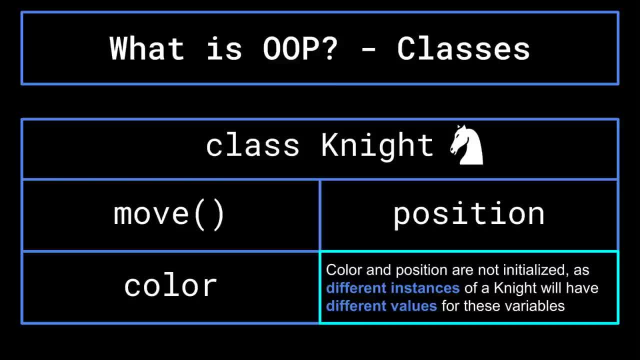 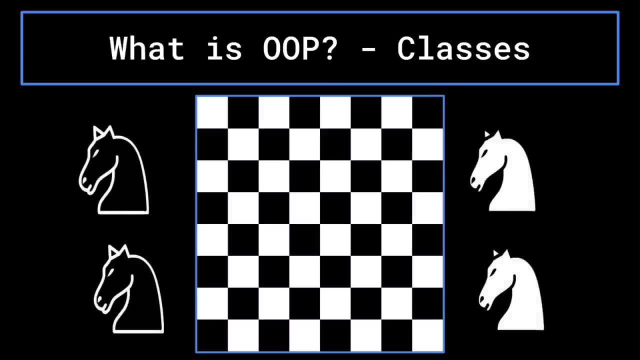 different data, for it's best to define them when I create the object rather than in the class itself. For instance, each of the four nights that begin in the game of chess start on different square than one another. Initializing the position variable in the night class would imply that 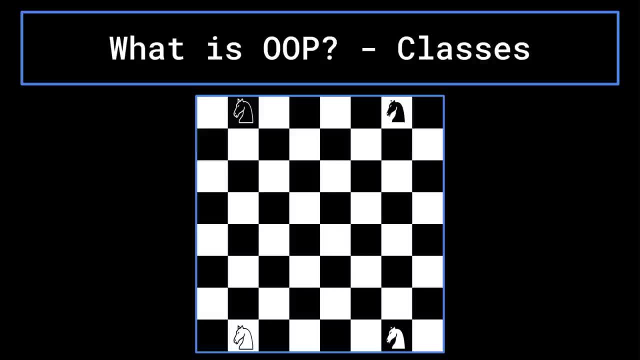 you want each night object created from this class to begin with the same position, which you do not. However, each of the nights would behave the same in terms of the squares that could move to, based on their position, And thus it is best to define a move function in the class rather. 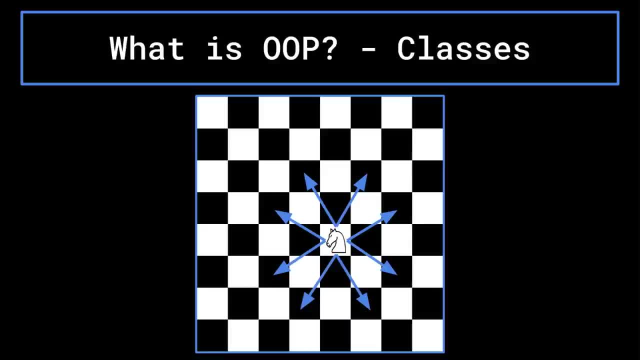 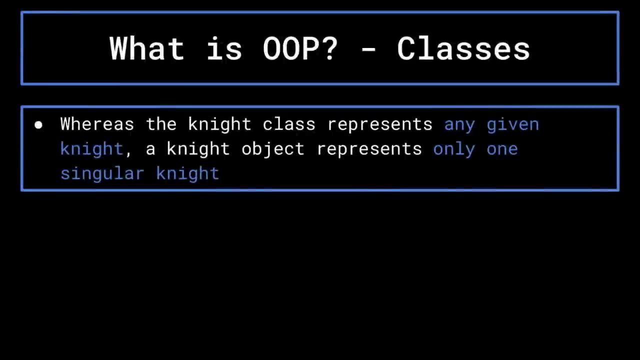 than repeating the same function definition in each object that I create. When creating a night object, you initialize its attributes or its variables and its methods or its functions to contain information specific to that night. Whereas the night class represents any given night, a night object represents one night in particular. 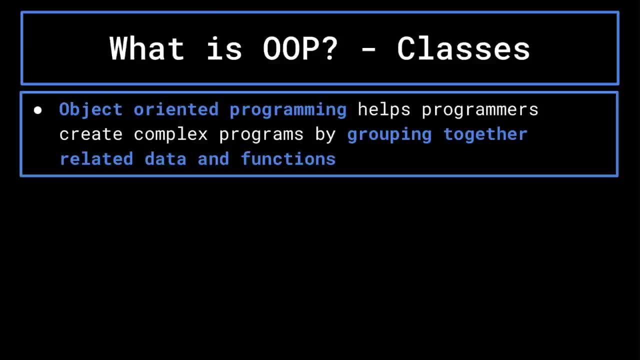 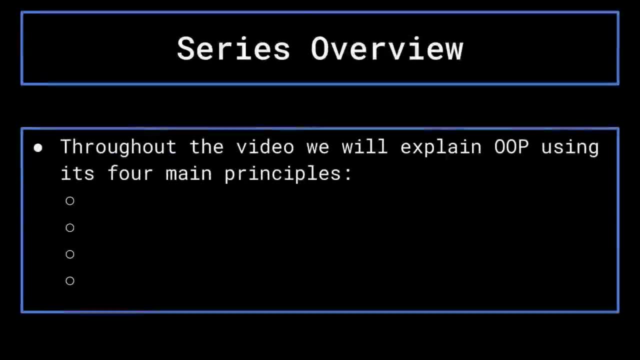 Essentially, object oriented programming is the best tool us programmers have right now to create complex programs by grouping together related data and functions. Throughout the course of this video we are going to be getting into detail into how all of this works, using the four main principles. 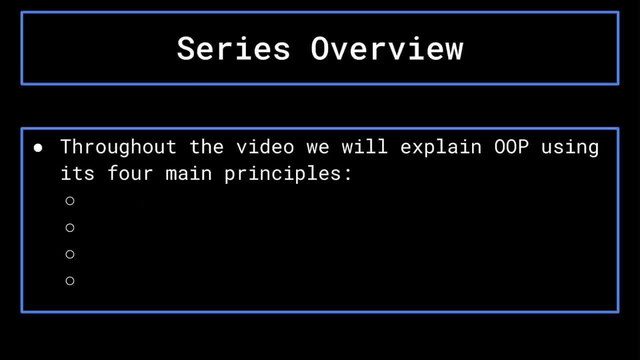 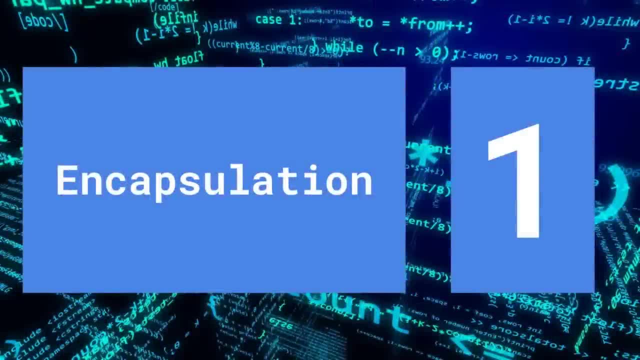 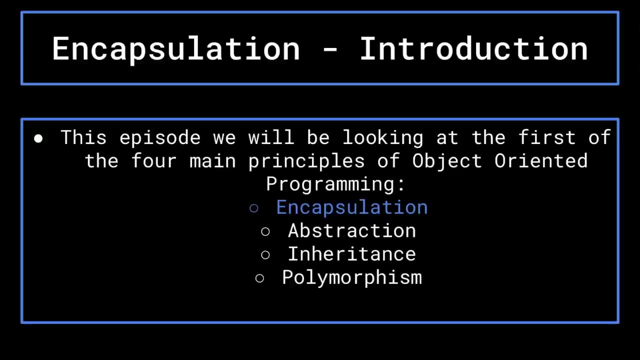 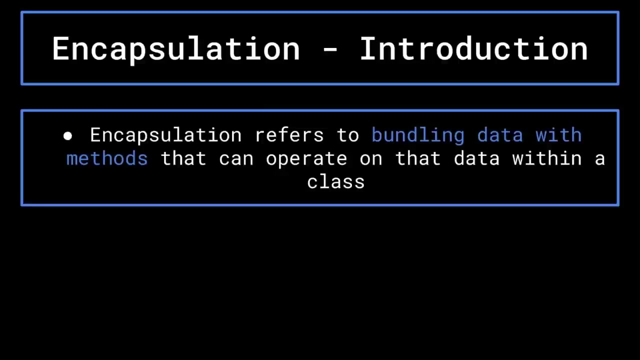 of object oriented programming, those being encapsulation, abstraction, inheritance and polymorphism. This next section is going to be focusing on the first of the four main principles of object oriented programming: encapsulation. Encapsulation refers to bundling data along with methods that can operate on that data. 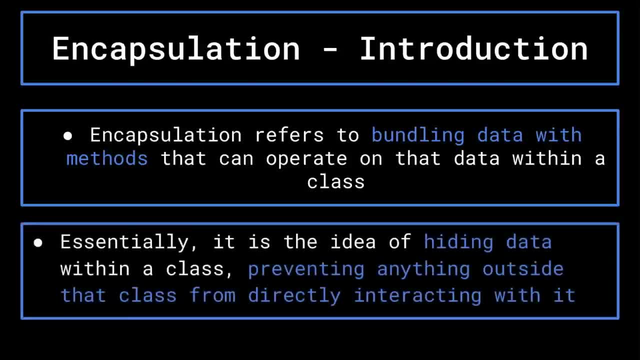 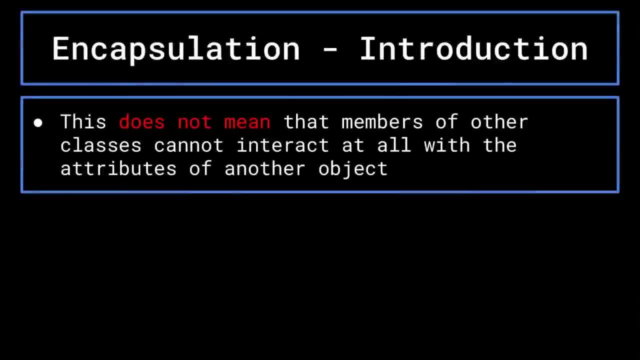 within a class. Essentially, it is the idea of hiding data within a class that anything outside that class cannot directly interact with. That is not to say that they are unable to interact with a separate objects attributes at all. however, instead members. 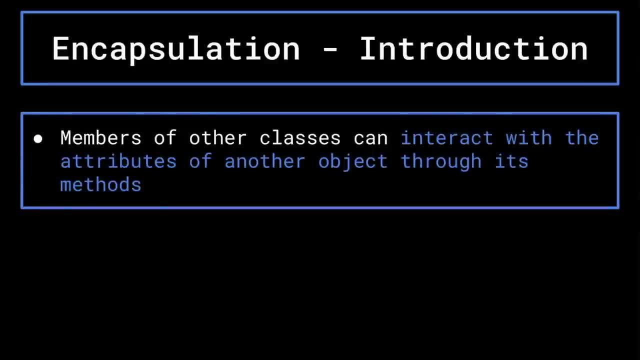 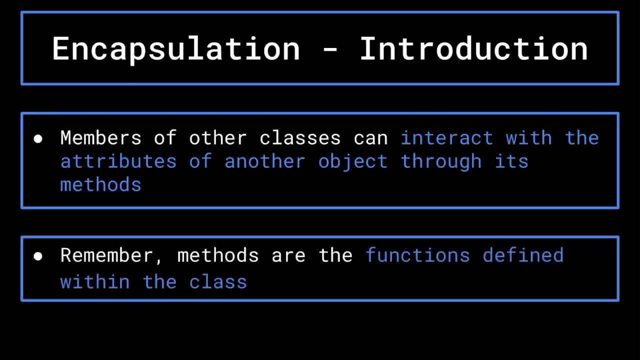 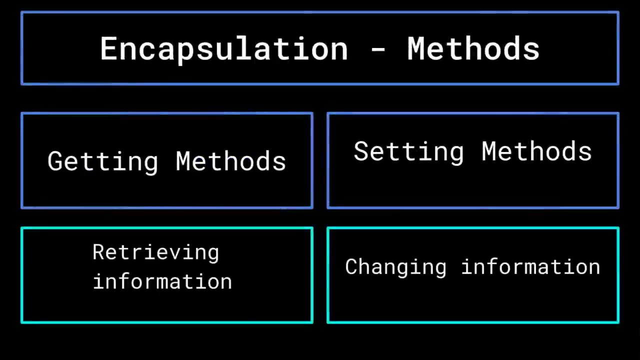 of other classes looking to interact with the attributes of an object should only be able to do so through that classes methods. In practice, one way this tends to work is by creating an object is by creating, getting and setting methods. These methods act to either get information- 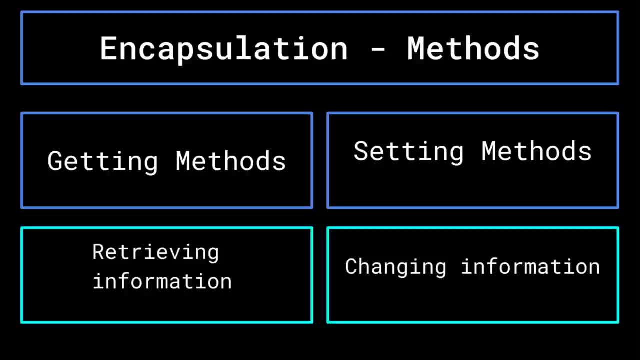 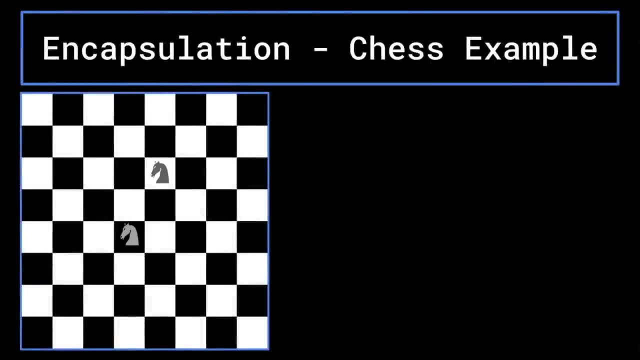 from an object or set attributes to different values, For instance. think back to the chess example from the previous section. If I was moving one piece and I wanted to determine whether it was able to capture another piece, I would need to define a dot get method associated. 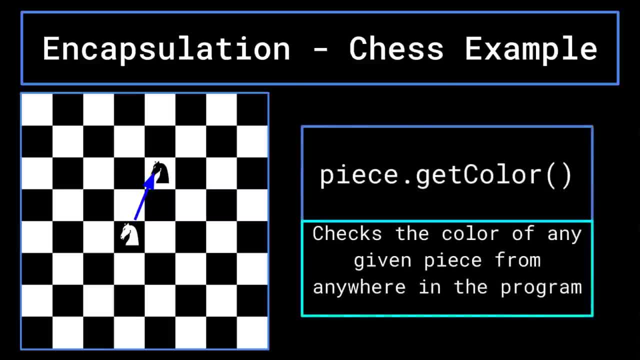 with each piece. that returns the pieces color. In this case, piece dot get color. This way, I could check the color of any piece from anywhere in my code without having to access the internal attributes of said pieces. This allows us to retrieve the information from where it is defined Additionally. 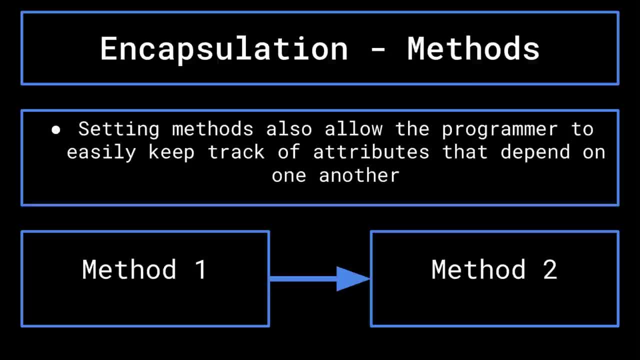 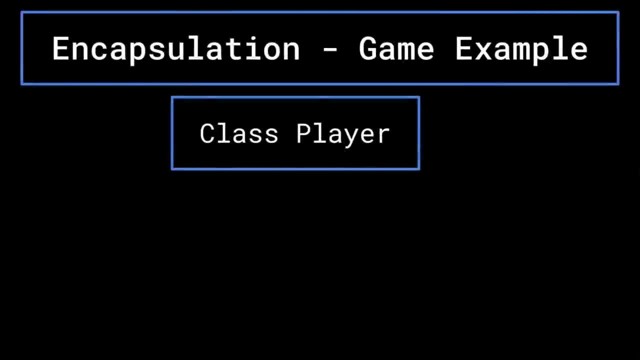 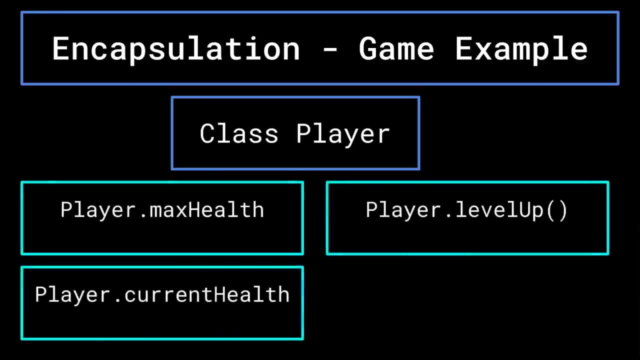 this makes it easiest to keep track of attributes that depend on one another. For example, if I was programming a game, I may have two different attributes for the player: self Max health and current health. When the character levels up, I may have their max health increase. 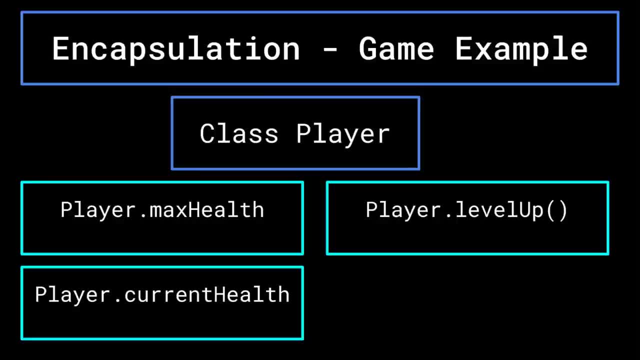 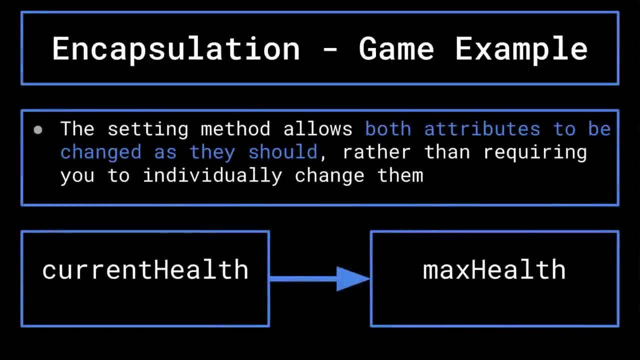 as well. When this happens, I would want the current health to be set to the maximum health. Instead of changing both of these values directly, I can define the set max health method such that the current health is also set to the maximum health once the maximum health has. 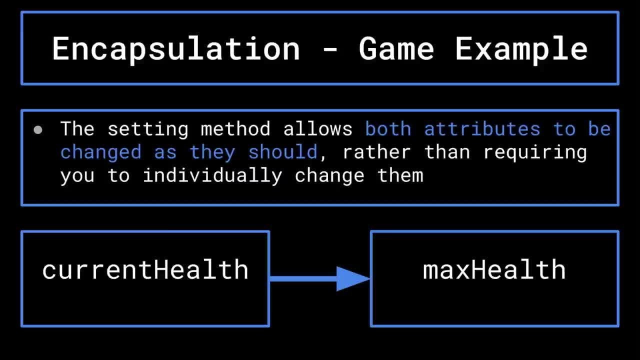 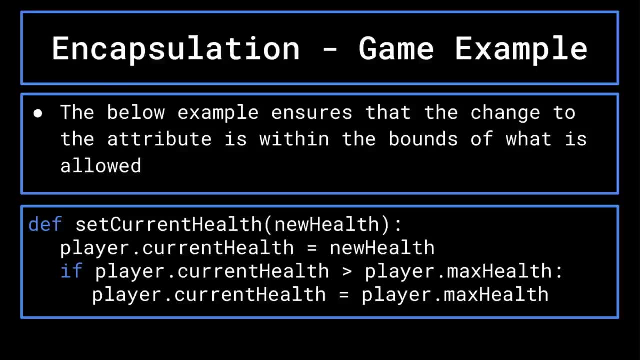 increased. Furthermore, these setting methods allow values to be validated. For instance, if current health is not able to exceed maximum health, then I would have the set current health method check if current health would be greater to maximum health before making the change. 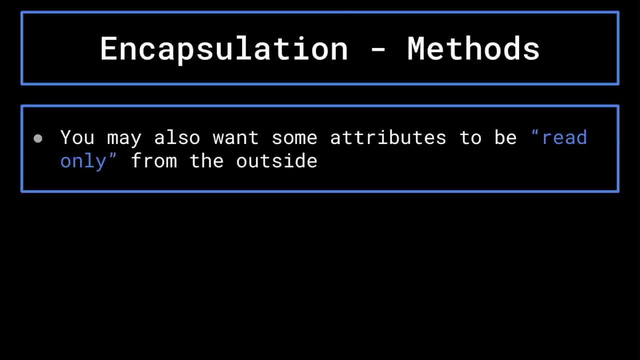 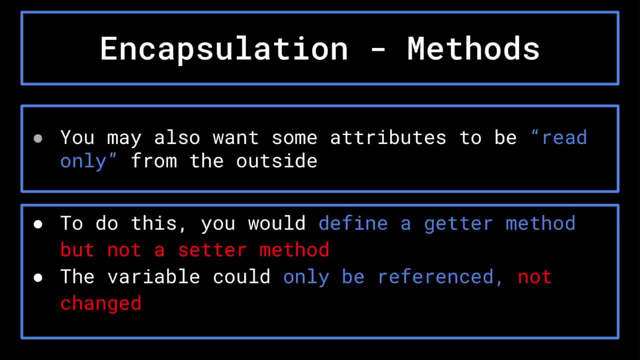 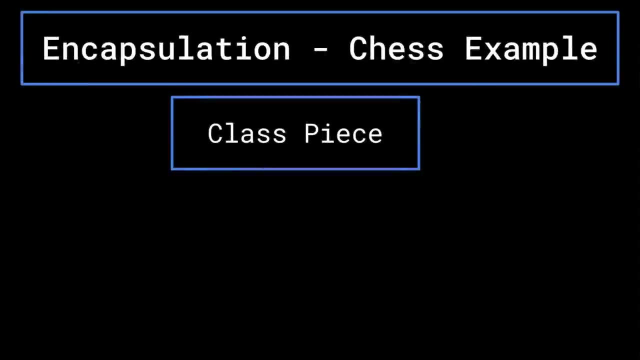 Finally, you may want some values to be read only from outside of class, which means you would only define a getter method and not a setter method. For another example, let's look back at chess. When dealing with a piece's position you would want to keep track of, 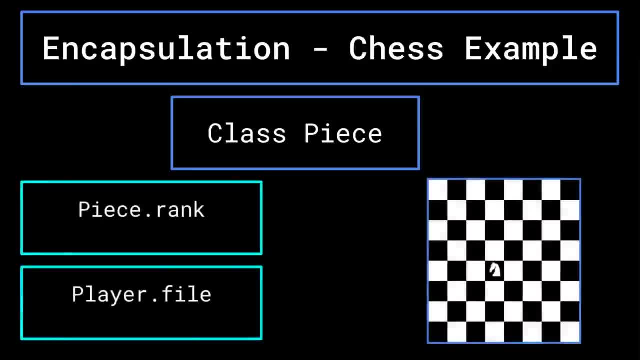 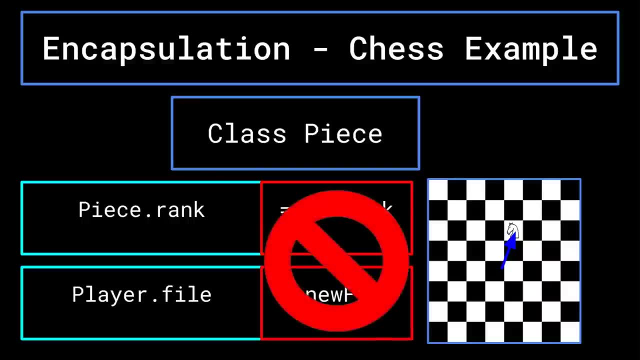 its rank or its row and its file or its column When the piece moves. you may think it would be okay to just set piece dot rank and piece dot file to new values. However, as discussed above, this is not the best way to handle it. It would be better to define a piece dot move function that 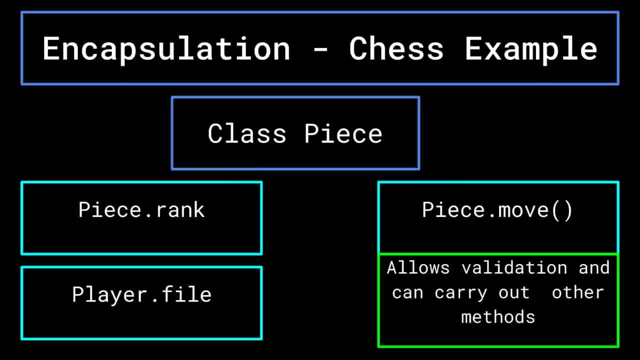 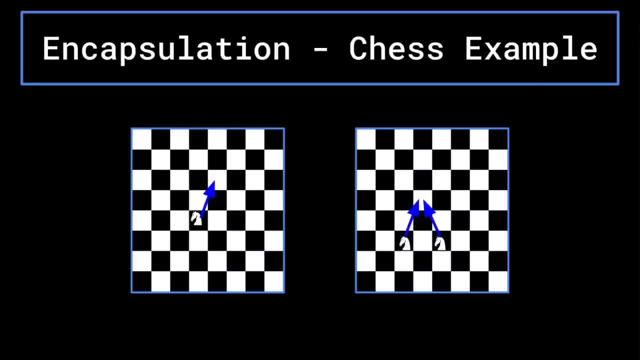 takes the intended new key to the new key. For example, if I want to set a new key to the new key, I would need to set a new position and checks if that is indeed a valid move. The piece would not be able to move if, say, the new location is off the board. a piece of the same color is already. 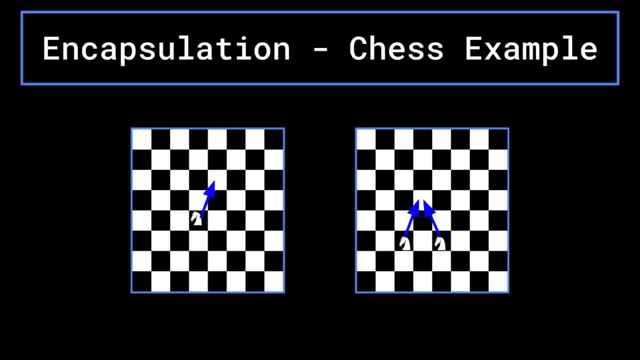 on that square, or making such a move would put the king of the same color in check. Additionally, other methods may be called from this move method, for instance, one that captures an enemy piece if it was on that square, or one that puts the enemy king in check, Were the piece's attributes just to. 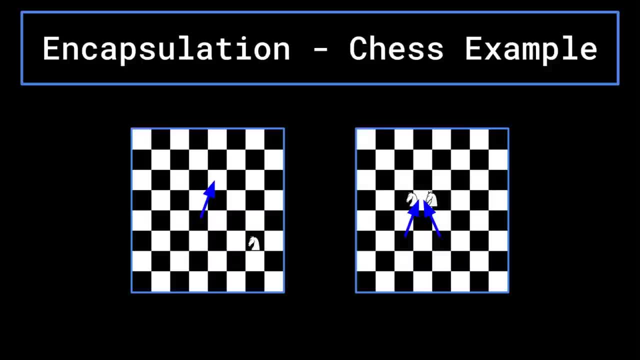 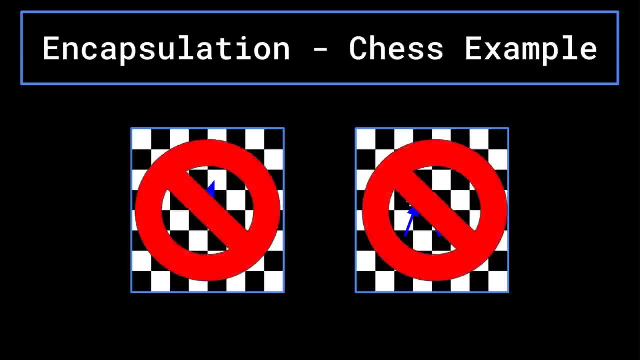 be directly changed. you could end up in a strange situation where illegal moves are played and pieces occupy the same square. Essentially, getter methods allowing validation can be very useful. Encapsulation is useful for a variety of reasons, As we just went over. it is best to not. 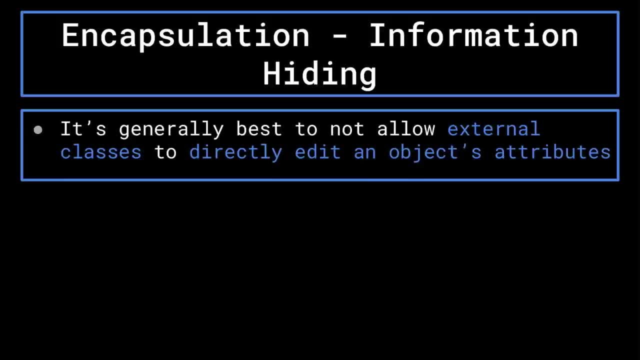 allow anything external to directly edit in objects attributes. This is especially true when working on large objects. For example, if you have a large object and you want to change its size, you may want to change the size of the object. For example, if you have a large object and 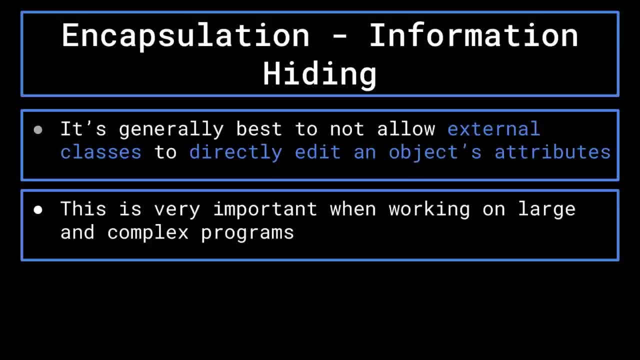 you want to change its size. you may want to change the size of the object. For example, if you have a large object and you want to change its size, you may want to change the size of the object, Individual pieces of the program to work well without requiring them to rely on every other. 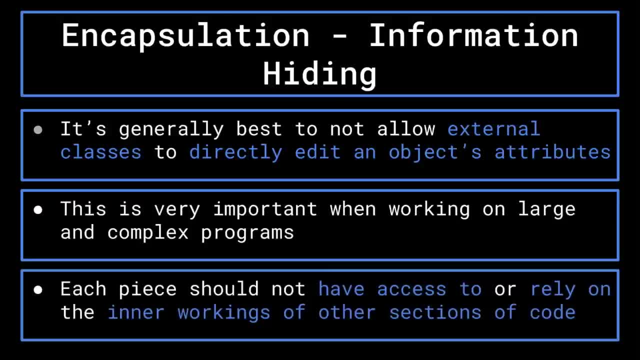 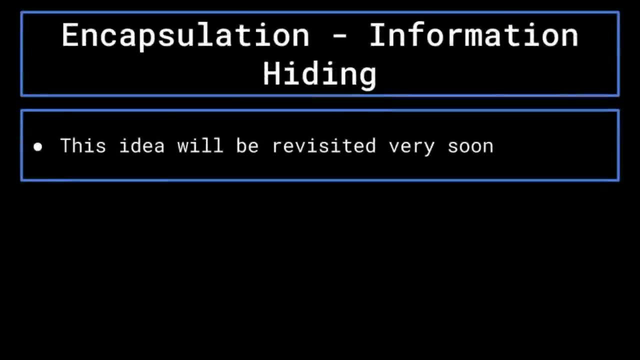 section of the code In this way, preventing each piece of your code from referencing and requiring knowledge of the inner workings of each other section of code is very important to keep your program from becoming completely entangled in itself. This is an idea we will touch upon in future sections to come, But for now, 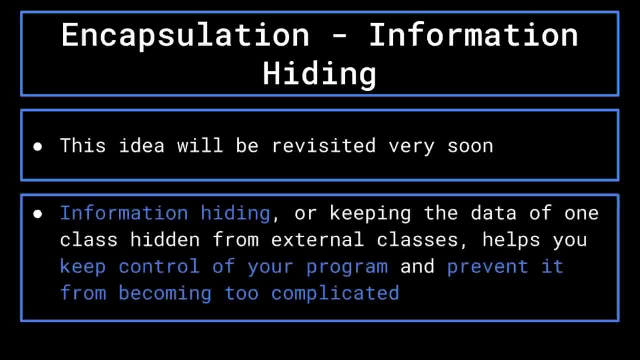 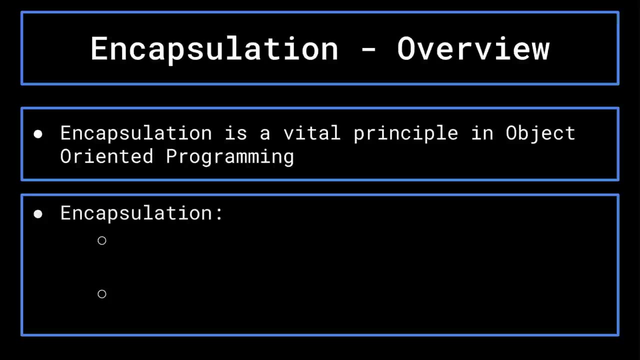 it's best to understand that information hiding- that is, keeping one class from being able to directly access the data of another class- is important to keep control of your program and reducing its overall complexity. Overall encapsulation is a vital component of object oriented programming. that allows the programmer to maintain control of their data and to keep 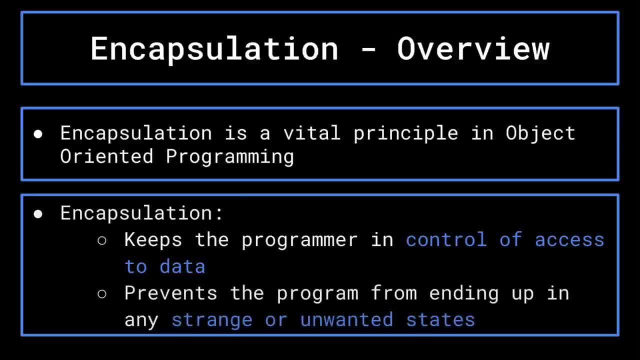 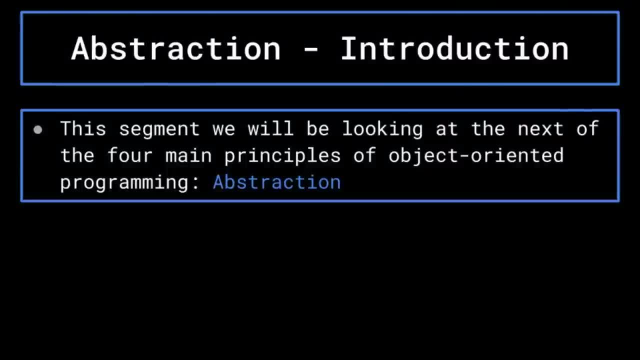 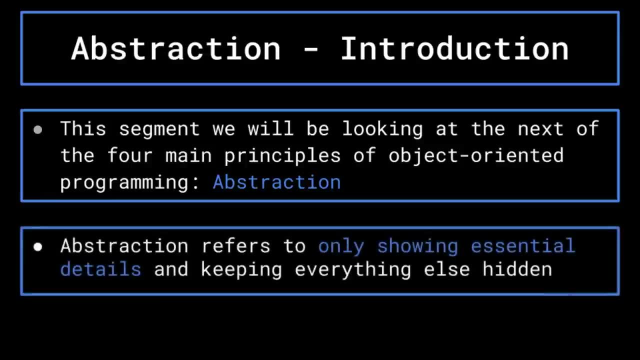 their program from ending up in any unwanted states. In this next section we are going to be discussing the next of the four main principles of object oriented programming: abstraction. Abstraction refers to the idea of only showing essential details and hiding everything else. This idea is present in everyday life. 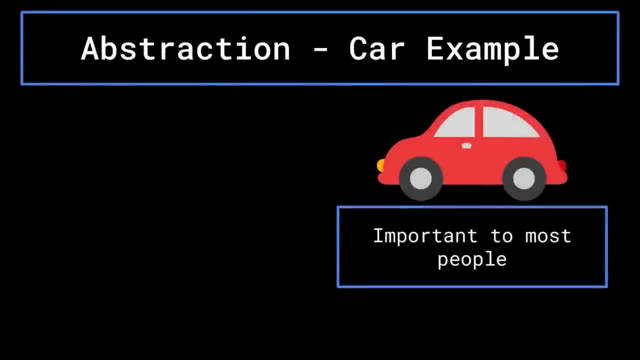 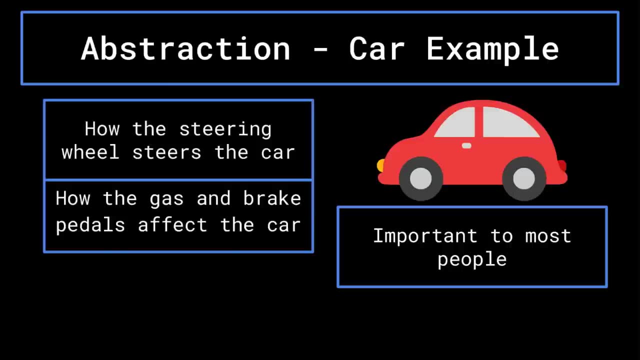 When you drive your car, there are some things you need to understand about it. You need to understand how the steering wheel steers the car, how the gas and brake pedals work. You also need to know how much gas your car has and that it needs gas to work. These are necessary details for you to be able to drive the car. 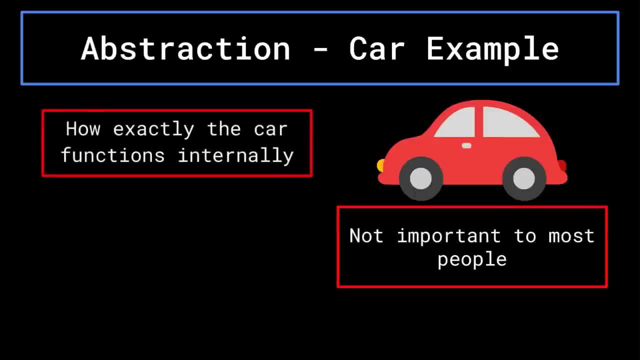 properly. However, the exact way that the car works internally isn't something that most people need to concern themselves with. How the gas reacts in the engine and how that translates into the car moving forward really isn't important while you are driving your car. 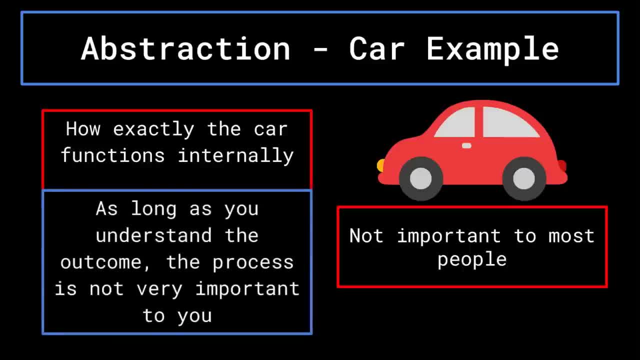 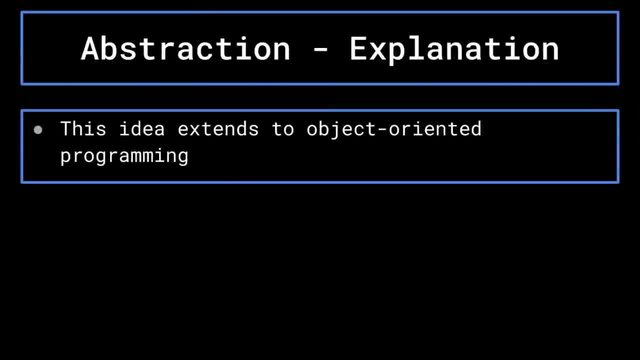 All that matters is that you know it will work this way. Whoever built the car had to worry about how exactly the car would work. so that you don't have to. This idea extends to object oriented programming. The classes you create should act like your car. 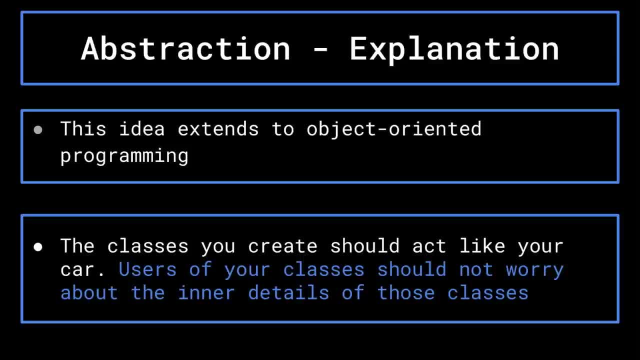 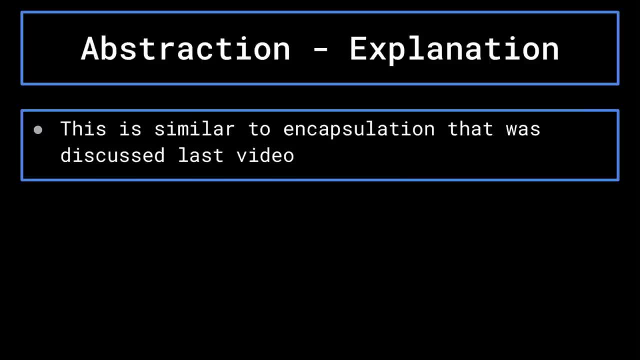 Users of your classes should not worry about the exact inner details of said classes. This idea is similar to that of encapsulation that we discussed in the previous section. Earlier, we mentioned how you should not have classes directly interact with the data stored within other classes. This idea is similar to that of encapsulation that we discussed in the previous. 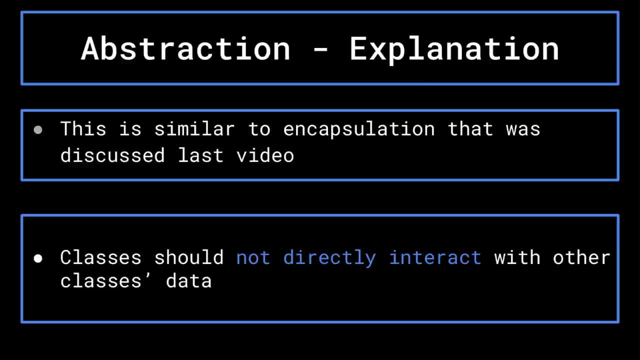 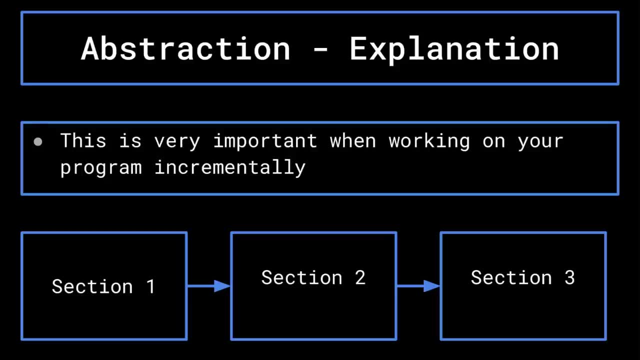 section, Rather have them use the classes' methods to access their data. This idea is especially important when you want to work on your program incrementally, where you focus on one class at a time and ensure that it works. This is a very useful approach. 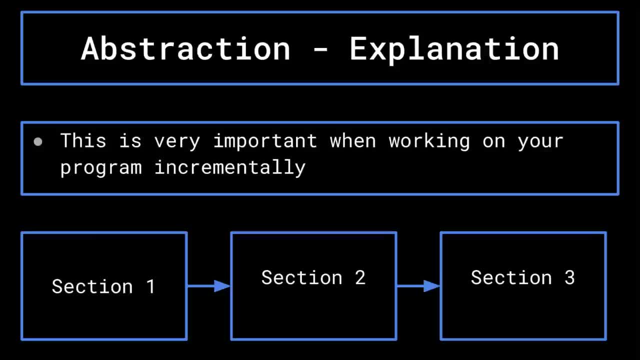 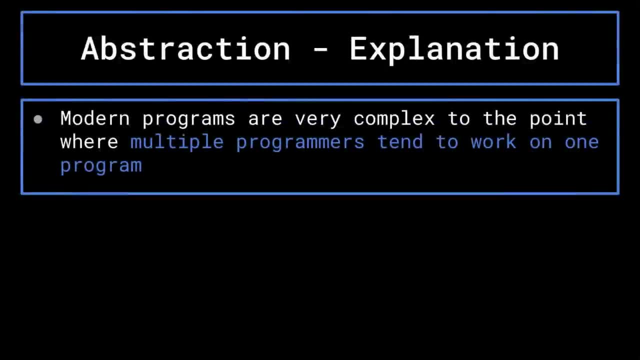 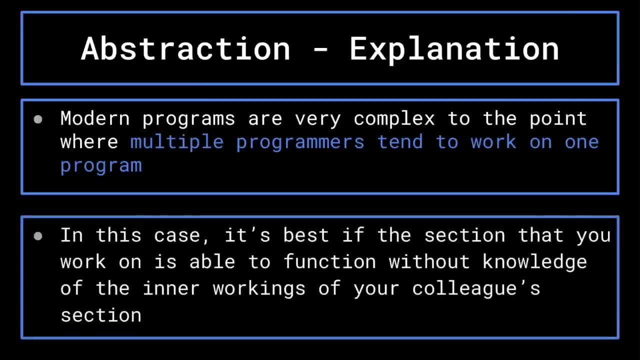 as it can be difficult for you to focus on the big picture while programming, and splitting up your project into smaller chunks can make it much more manageable. Furthermore, programs nowadays are vast and complex, to the point where multiple programmers tend to work on one project. In this case, it's best if the section that you are working on is able to 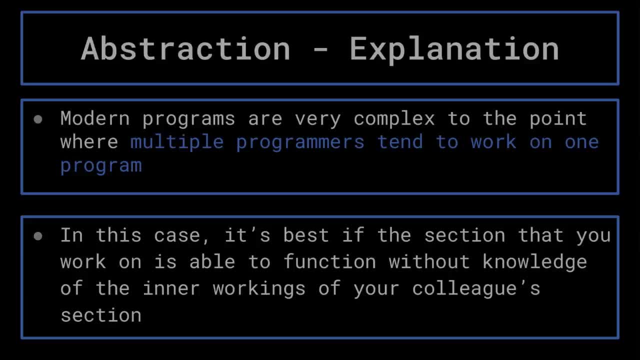 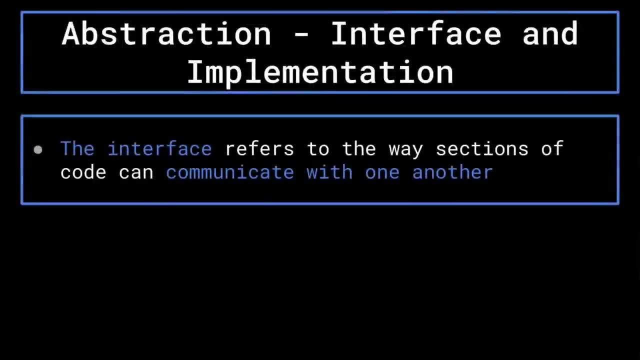 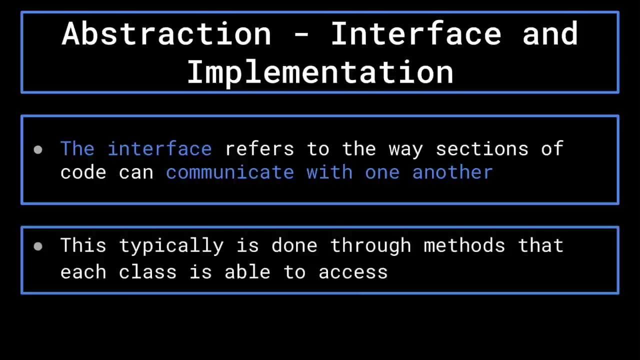 function without knowledge of the inner workings of your colleague section. To achieve this, it's best to think of your program in terms of interface and implementation. The interface refers to the ways that sections of code are able to communicate with one another. This is typically done through methods that each class is able to access The exact implementation. 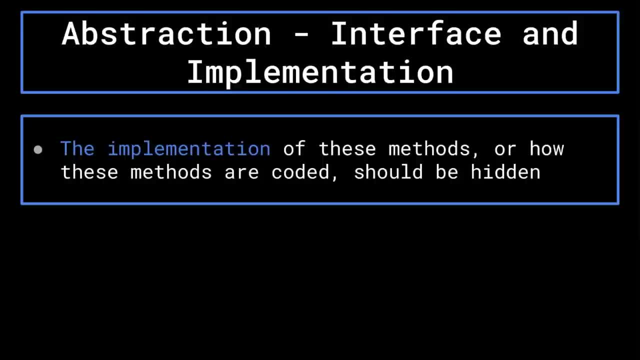 of these methods, or how the methods are coded, should be hidden within the class and not accessible from the outside. Think of this: like the car, The other classes are able to turn the wheel and push the gas, and they know what the outcome should be without caring about exactly. 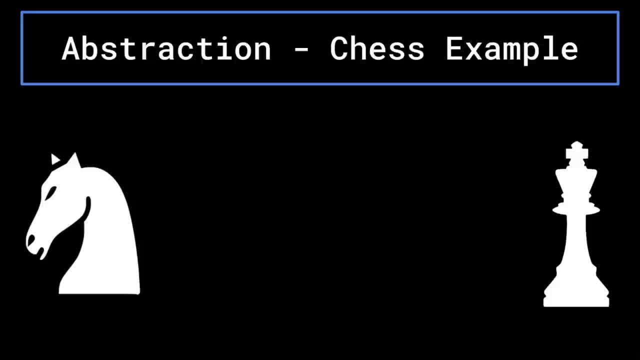 how this gets done. Let's return to the chess example that we've been using throughout the video. Let's say that you are working on making the knight work as it should and a fellow programmer is working in the king class. In order to effectively work together, you need to agree on an interface with which these pieces 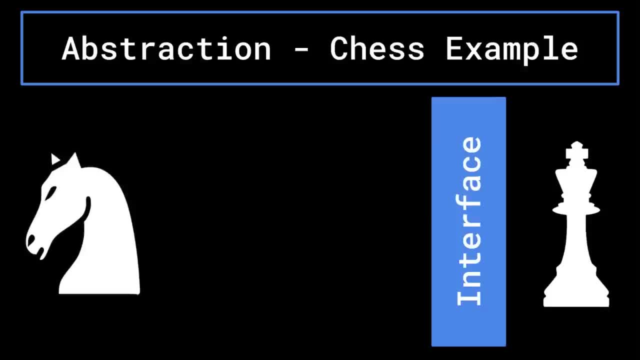 are able to communicate. In this case, say that you are working on making the knight unable to move if your king is in check. As the programmer of the knight class, you make the knight use the king's getter method. that will let the knight know whether or not the king is in check, If it is. 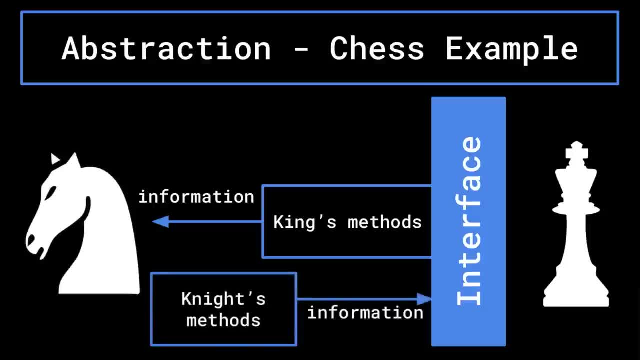 then you make it so the knight is not able to move unless it is able to put the king out of check. As you program the knight class, you should not be concerned with how the king is determining whether or not it is in check. The king's method that tells the knight 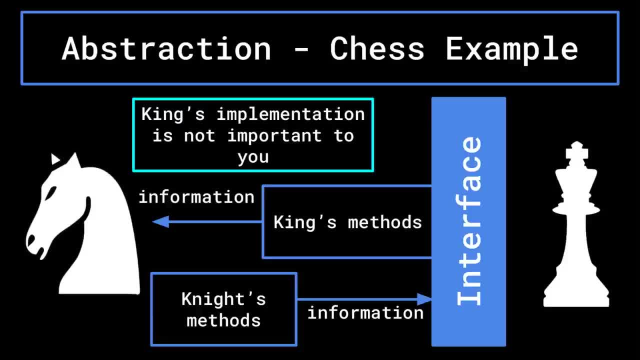 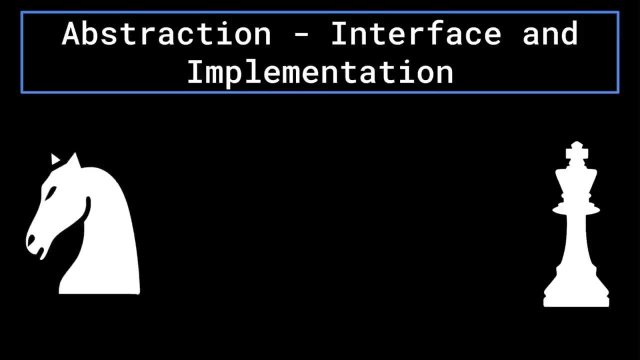 whether or not it is in check is part of the interface, but how exactly it does that is part of the implementation. This manner of only allowing the classes to interact through a predetermined interface prevents different pieces of the program from becoming completely coupled together. If the knight class has to look into the king class in order to make a determination, 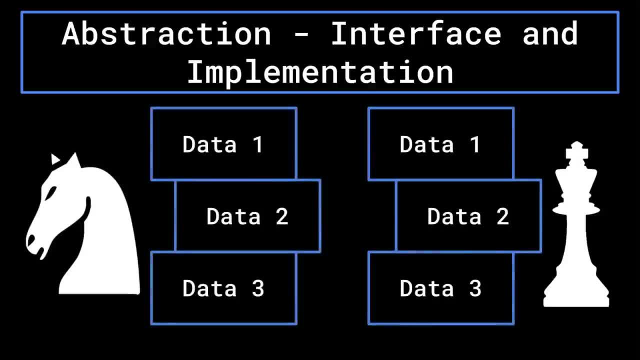 then it is reliant on the king class being set up in a certain way in order to function. If the king class is changed or reorganized or its data is renamed, then the knight class would no longer work and it too would have to be changed. 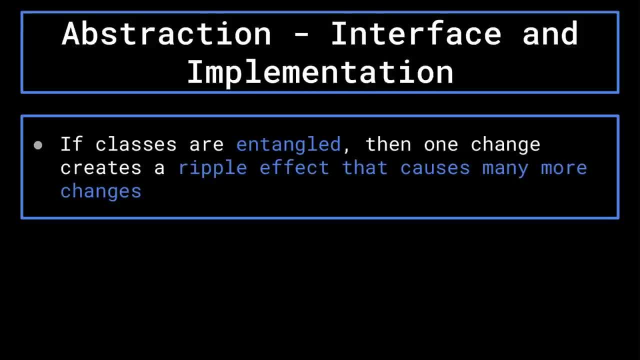 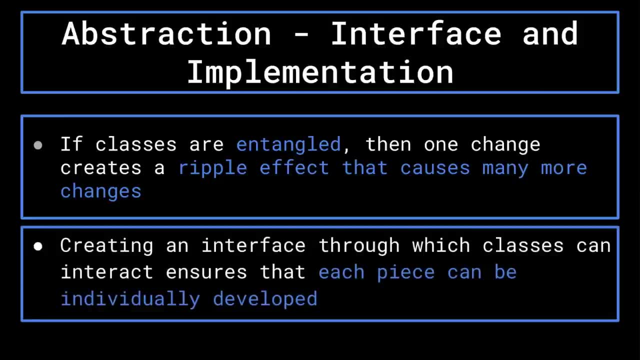 Assuming the rest of the program was coded in this way, then many other classes would also have to be modified. That interface, through which classes can interact with one another, ensures that each individual piece can be changed without creating a ripple effect that causes the entire program to have. 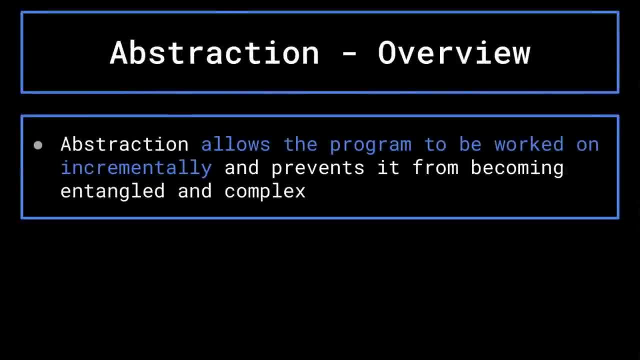 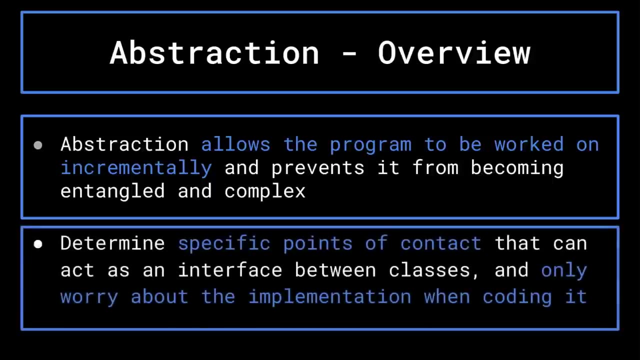 to change in response. Overall, it's best to keep in mind abstraction when writing object-oriented code, as it allows the program to be worked on incrementally and prevents it from becoming completely entangled in itself. and very complex Determine specific points of contact that can be. 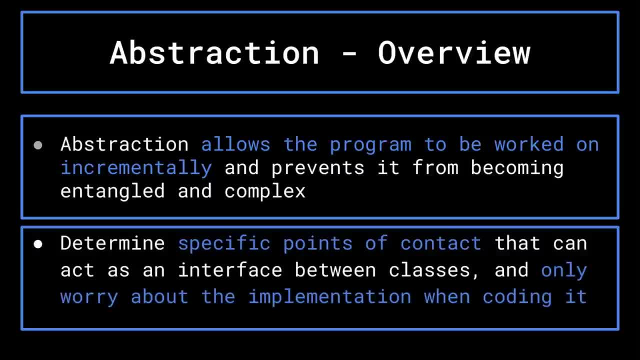 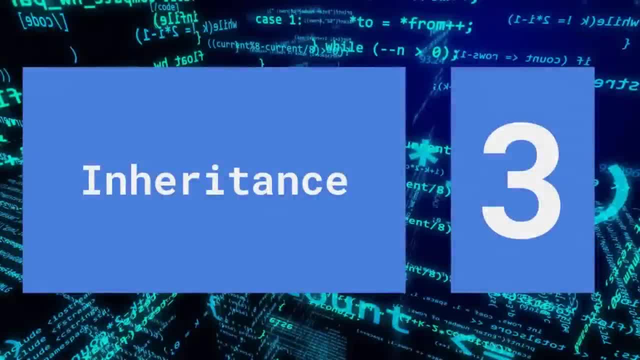 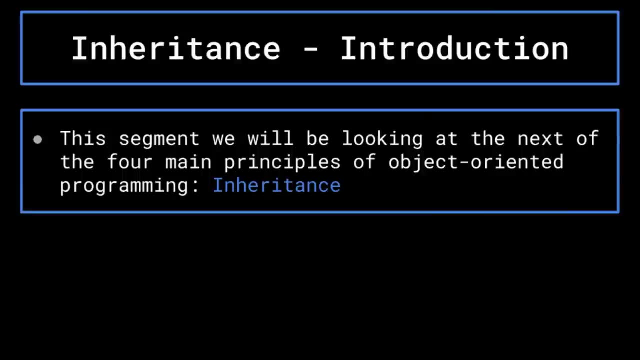 added to the interface between classes and only worry about the implementation behind it when working on that section. This next section will be tackling inheritance, the third of the main principles of object-oriented programming. Inheritance is the principle that allows you to derive classes from other classes. 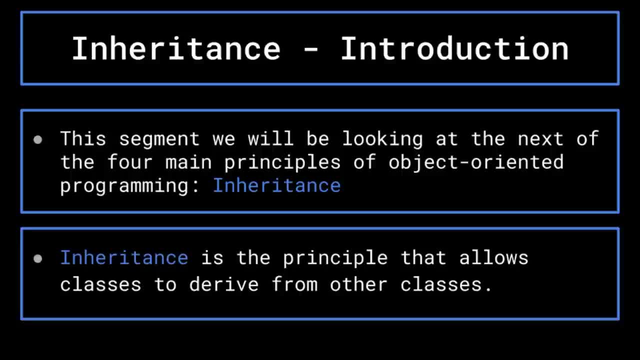 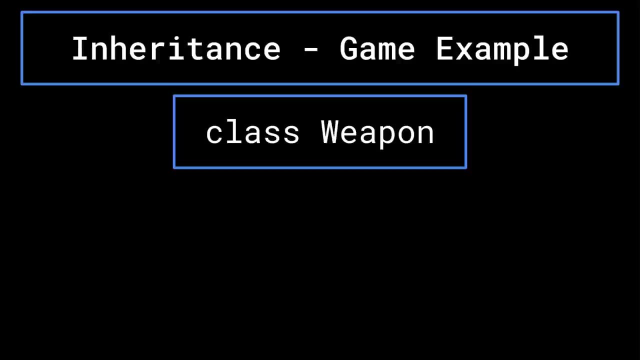 Classes can inherit certain methods and attributes from another class. We will get into exactly what this means in a moment, but first let's look at an example. Let's say you are programming a game. In this game, the player has access to weapons to fight. 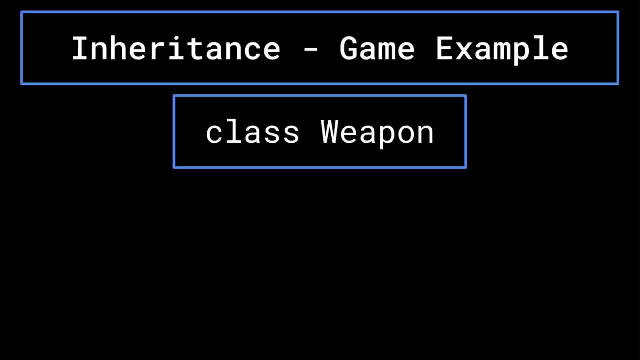 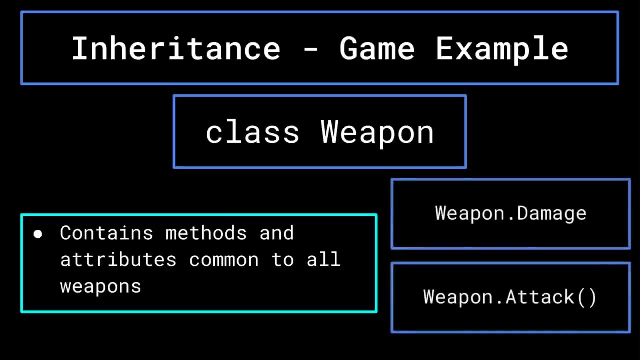 their enemies. To begin, you may establish a weapons class. This class would contain many of the pertinent attributes and methods common to weapons, for instance, an attribute that represents the damage that the weapon deals and a method that deals damage to an opponent when. 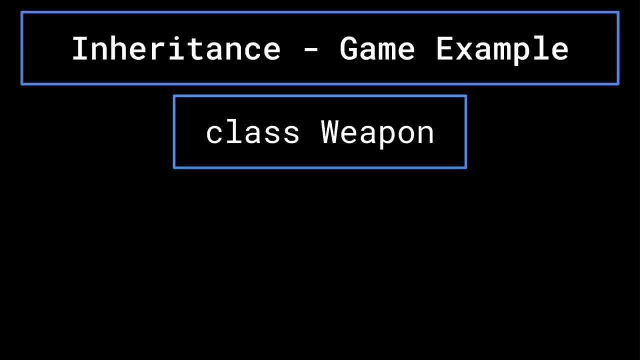 called You then, would want some more classes to represent specific weapons such as a sword or a club. These classes would act differently from one another, as swords and clubs have certain different attributes, such as a sword being made for cutting, whereas a club is blunt. 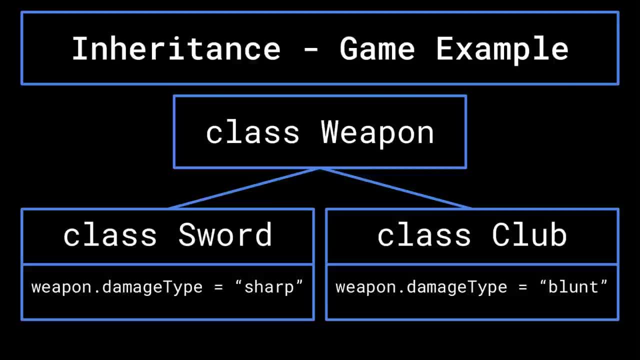 These differences would be represented in different values for their attributes, as well as possibly different attributes altogether. However, they do share much of the same behavior, as they are both members of the weapons class. In this case, the weapon class would be the. 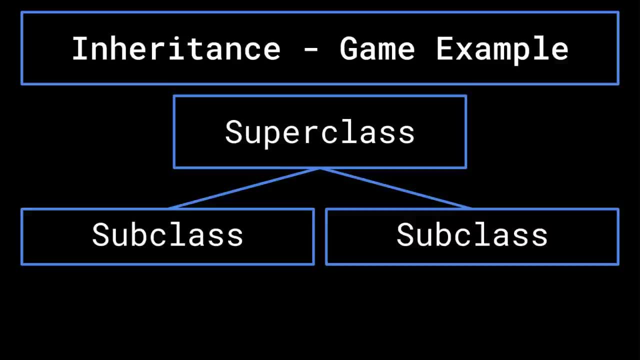 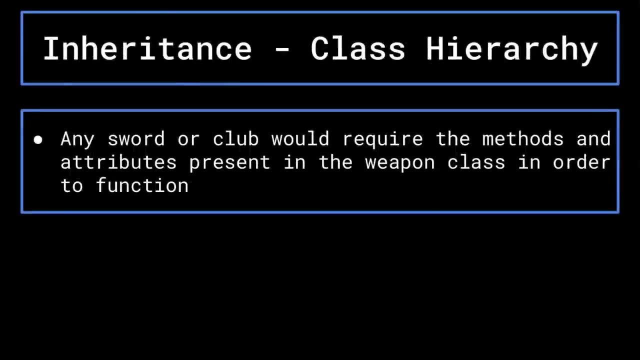 superclass, and the sword and club classes that extend the weapon class would be subclasses in relation to it. Many of the attributes and methods associated with the weapon class would also be present in its subclasses. Any given sword or club would also want access to the methods that allow them to deal damage. 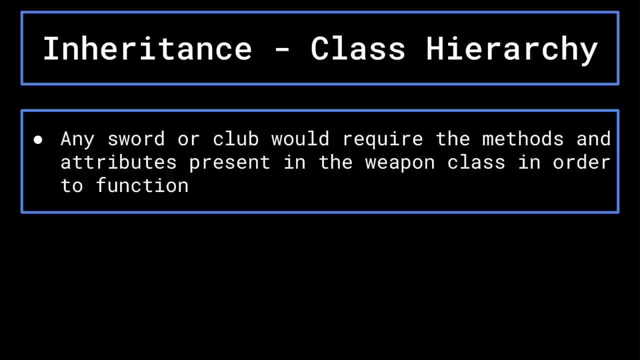 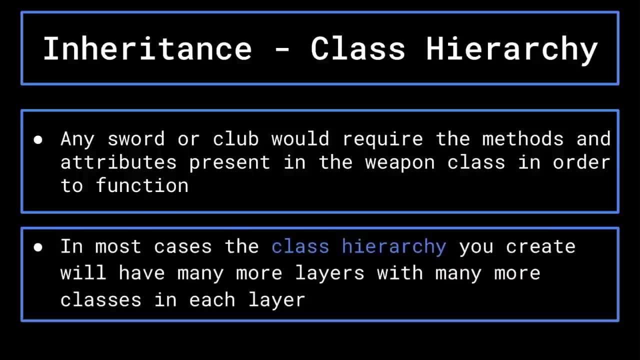 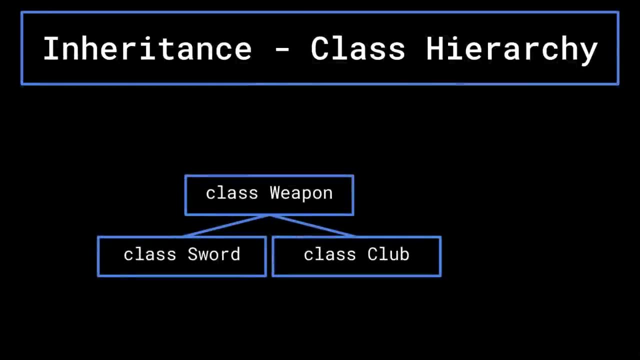 as well as the attributes that detail how much and what type of damage they deal. The class hierarchy does not tend to be so small, however, as in most cases there are many more layers than just one superclass and a couple of subclasses. The weapon class may be a subclass to. 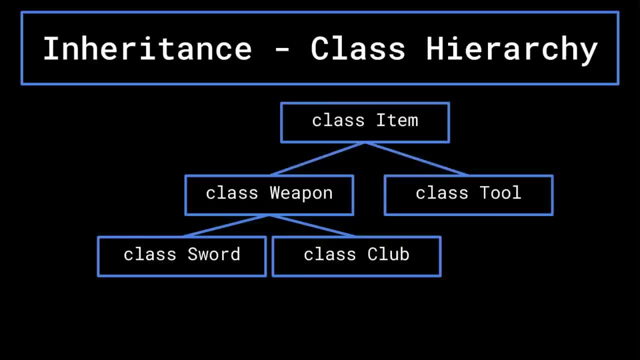 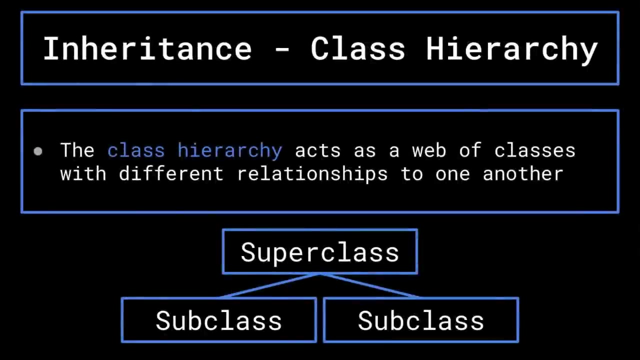 a broader items class which could contain many other subclasses with subclasses of their own. Additionally, you may include a wider variety of weapons than just swords and clubs, As well as multiple types of swords that would require different behaviors and thus their own subclasses. When you are writing object oriented code, many of the classes you create will fit. 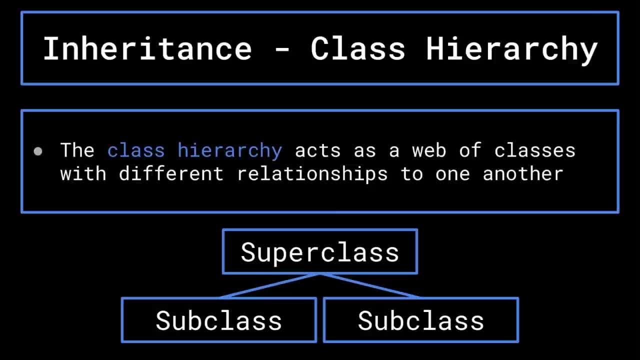 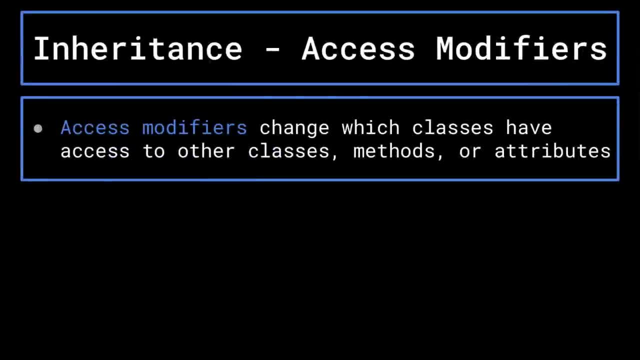 somewhere in the broader class hierarchy, which acts as a web of classes with different relationships to one another. The next important topic to cover in terms of inheritance is the access modifiers that change which classes access. which access modifiers If you have access modifiers which attributes methods or even classes as a whole. There are three main access modifiers. 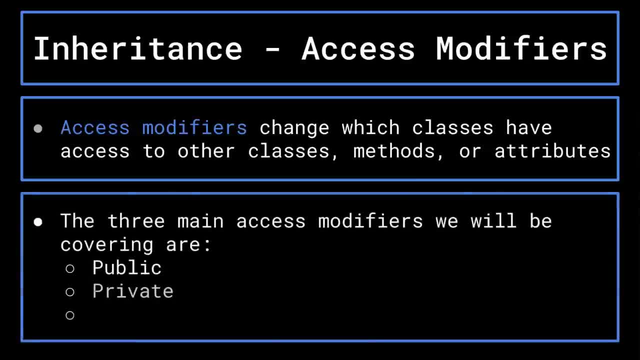 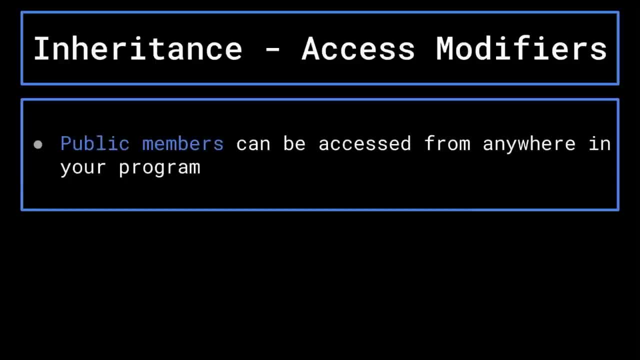 that we will be discussing public, private and protected. Let's begin with the public modifier. Public is probably the most simple of the modifiers. A public member or class can be accessed from anywhere. This includes any super classes, subclasses or anywhere else in the program. 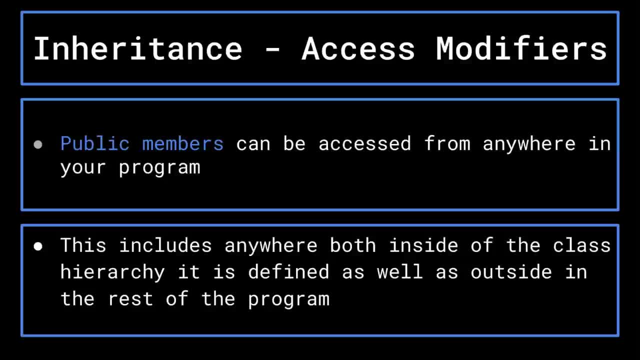 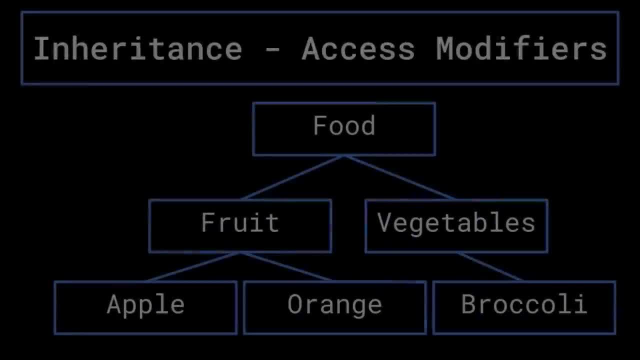 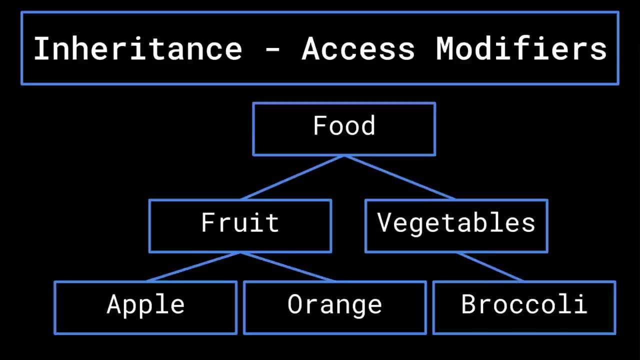 This is very useful when you need to have access from a wide variety of places in your program To better understand this modifier and those to come. look to the example class hierarchy on screen that represents different foods For each example. the member in question will be defined in the fruit class. 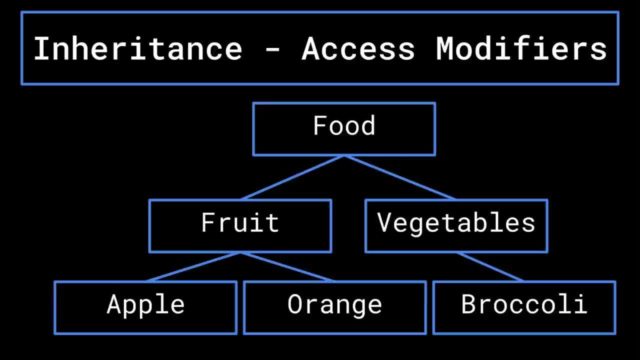 Green classes have access and red classes do not. As you can see, a public member being defined in this class or anywhere else in the program is not a public member. This means that a public member is followed by a private member. If another public member is made, they can indicate or take access. 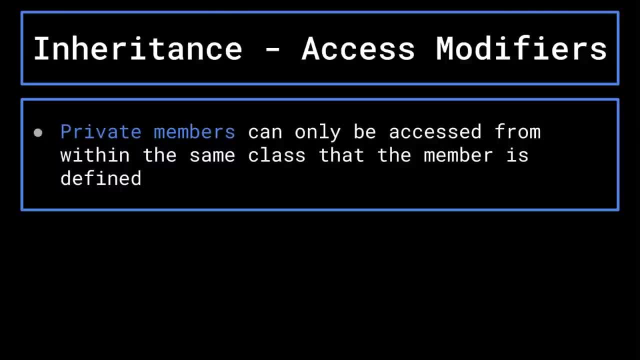 to any class within the same class by a subclass. Take the example first. a private member is tracks all of the members in a single class. If the public member is anybody destroying in any of the three classes, that is assigned to them, which is very easy for any member to not to use. 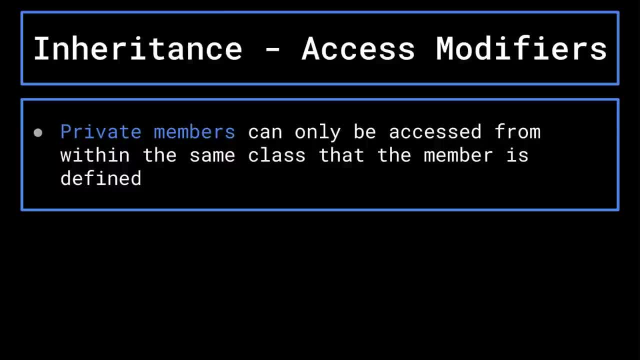 this information. separate classes that are assigned to any type of members will not use this information. These are the general options you'll see in your app. support cad allowed. Public members can also be unlocked within a single class, However private and not any type of members. can also be axis assigned to any member. This may require this to 不能 and you can also ask for additional reasons. If all of your members are in this, anybody class, including a member within a class, or any class, then the right points will be created to the. 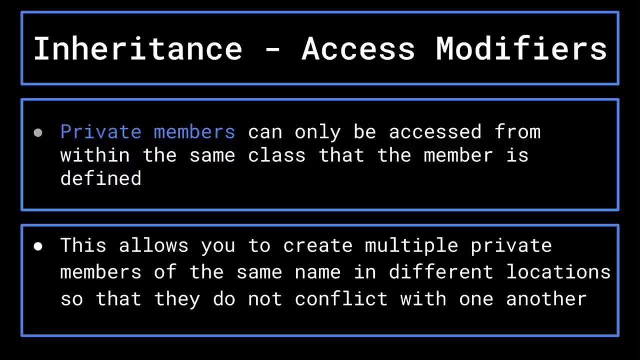 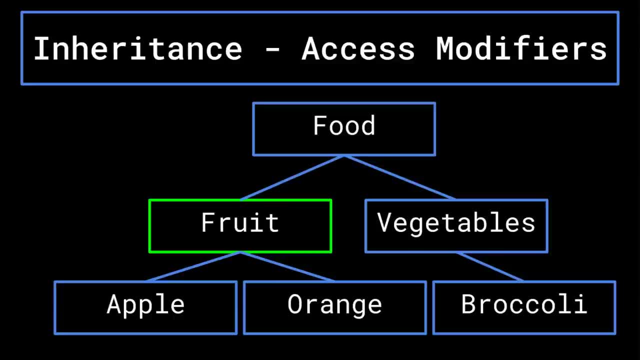 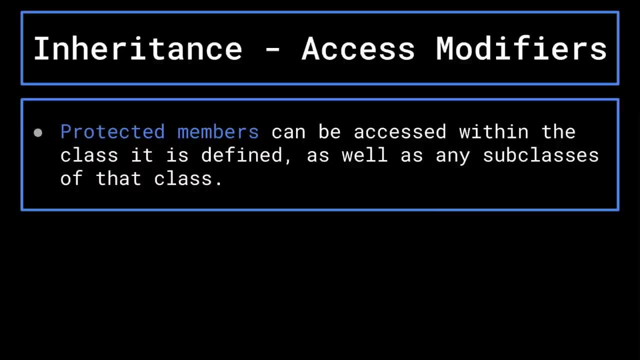 conflict with one another due to their private access modifier. As you can see on the example class hierarchy, a private member defined in the fruit class can only be accessed inside the fruit class. We then have the protected modifier. a protected variable can be accessed from within. 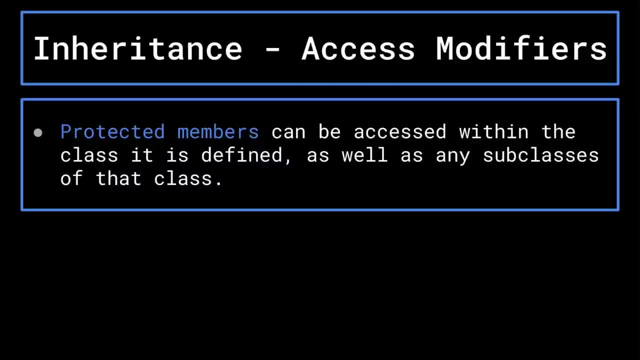 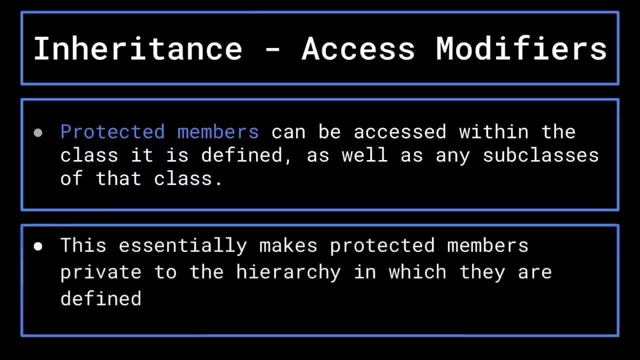 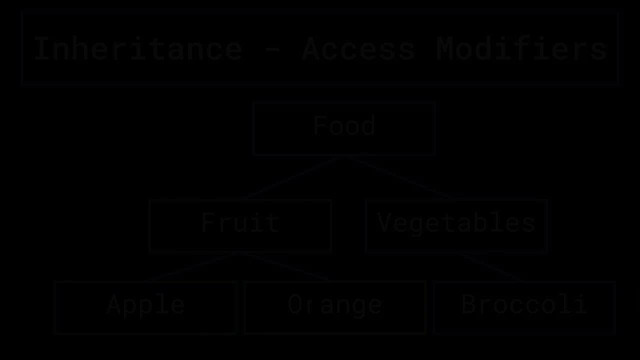 the class it is defined, as well as any subclasses of that class. Essentially protected variables are private to the class hierarchy that they are defined in. This can be seen in the example class hierarchy. right now In this final section, we will be covering the final of the four main 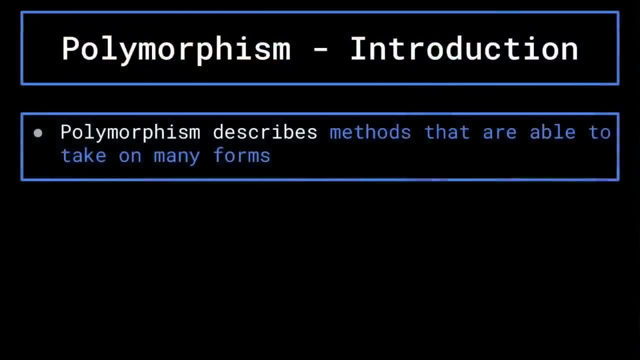 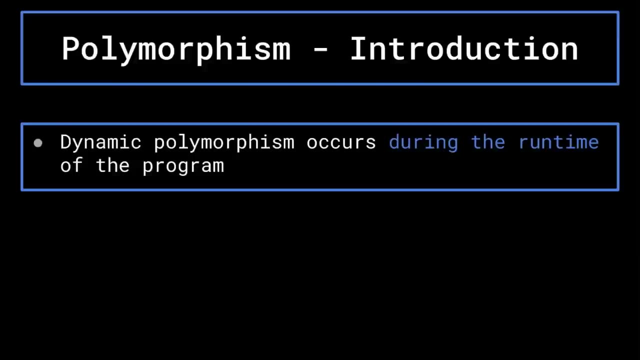 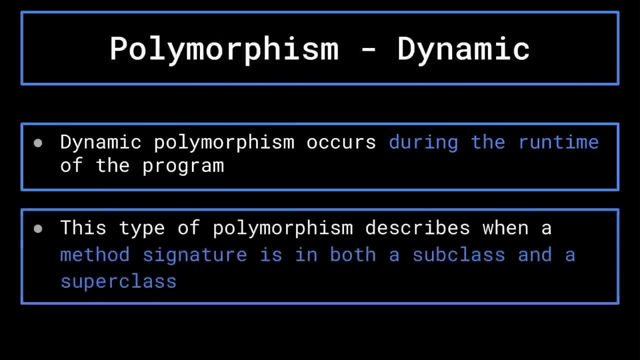 principles: polymorphism. Polymorphism describes methods that are able to take on many forms. There are two types of polymorphism. The first one is what is called dynamic polymorphism. Polymorphism occurs during runtime, when the program is being executed. This describes when a method signature 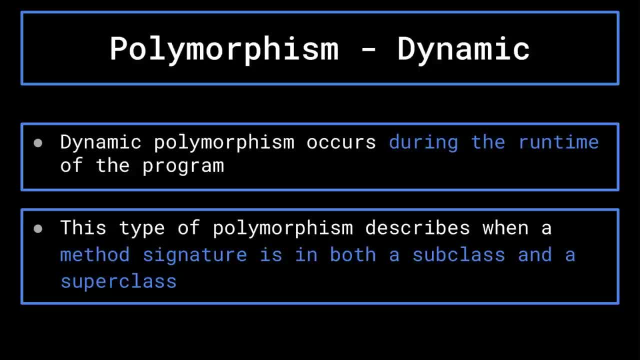 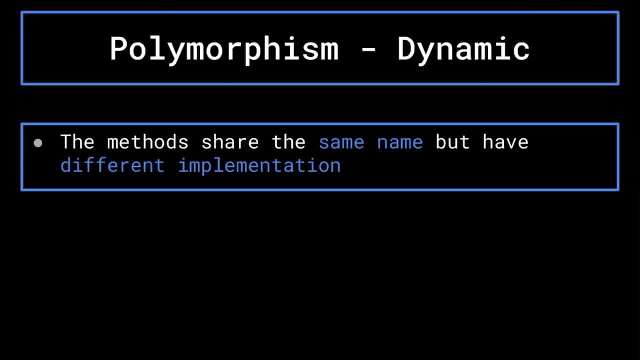 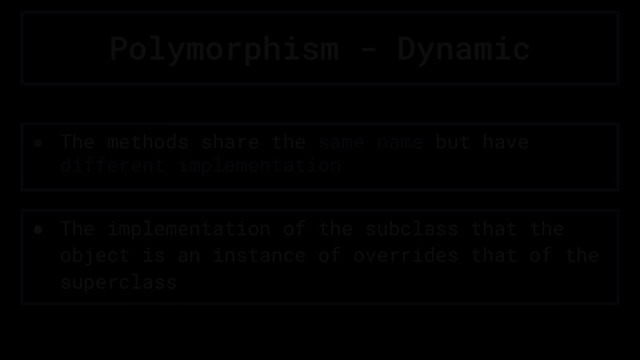 is present in both a subclass and a superclass. The methods share the same parameters but have separate implementation. In this case, the subclasses implementation of the method overrides the superclasses. Let's go over an example. Let's say you are running a program that uses the. 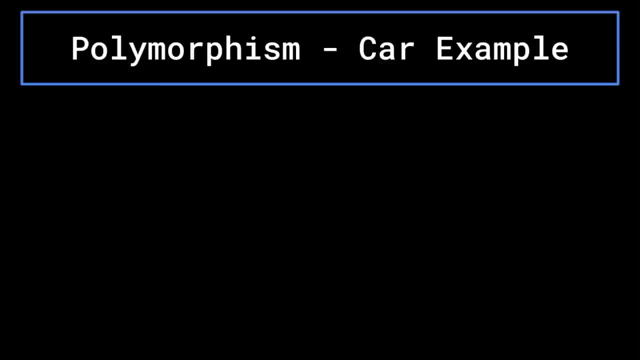 program. You are running a program to represent many different types of cars in a class hierarchy. At the top of the hierarchy you may have the generic car class. you then may create a sports car class as a subclass of the car class. you then may create a dot drive method. 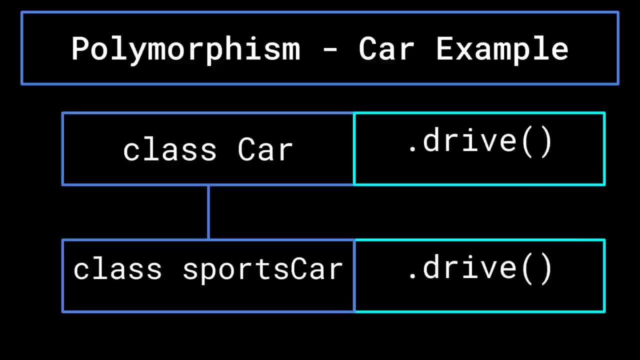 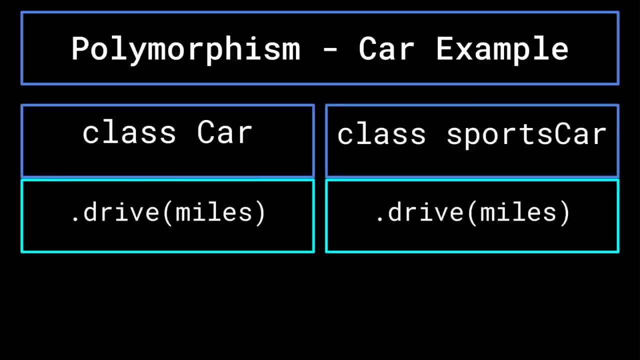 in both of the classes. In each of the classes, the dot drive function will take a double, representing the number of miles you would like the car to drive, And the cars gauges attribute will be decreased by the pertinent amount In the car class, the dot drive function. 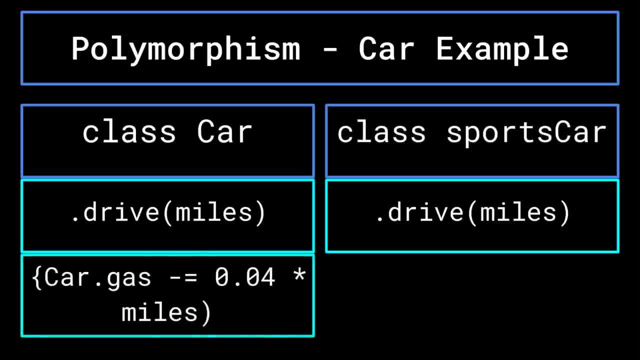 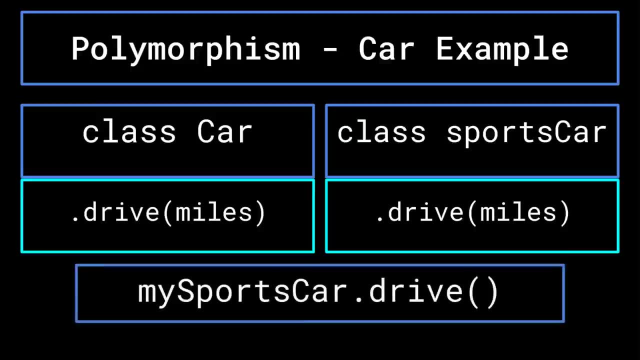 may cause the car's gas to decrease by 0.04 gallons per mile, whereas the sports car class may instead have its gas decreased by 0.02 gallons per mile. with drives, If you create an instance of a sports car called my sports car, the sports car implementation of the dot. 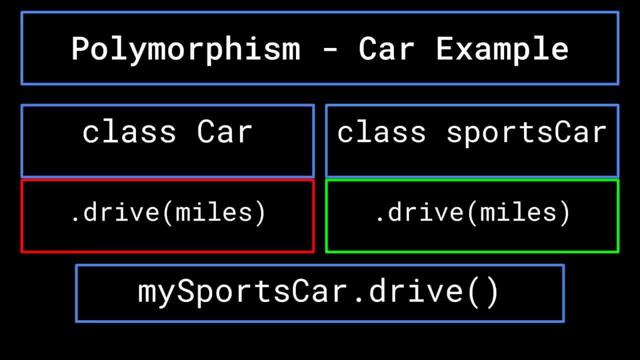 drive method will override the generic car version of the dot drive method. Therefore, my sports car dot drive will decrease my sports cars gas attribute by 0.02 gallons per mile. However, were you to create an instance of the car class called my car, my car dot drive would. 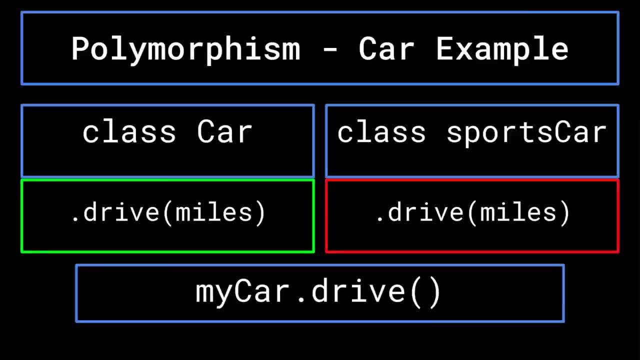 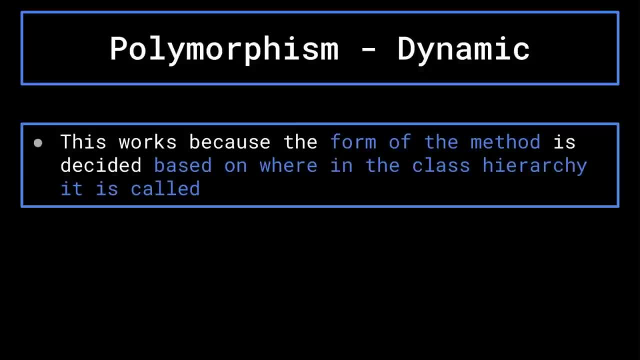 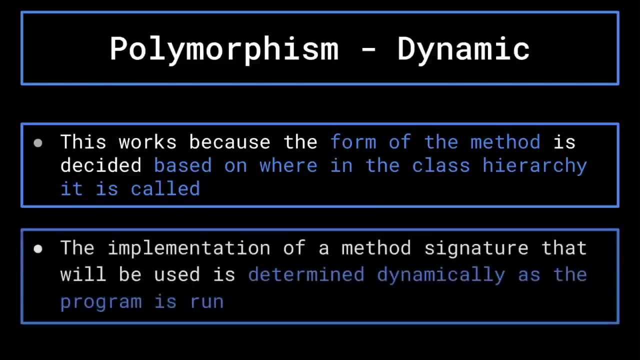 instead decrease my cars gas by 0.04 gallons per mile. This is an example of dynamic polymorphism, as the implementation of a method signature can change depending on which level in the class hierarchy that it is called. This works this way because the form of the method that is called is decided dynamically as the program is run. This idea 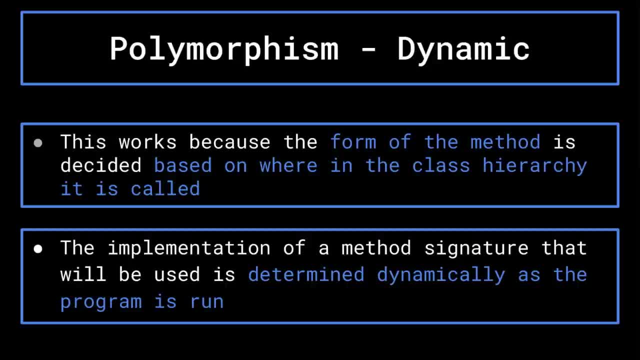 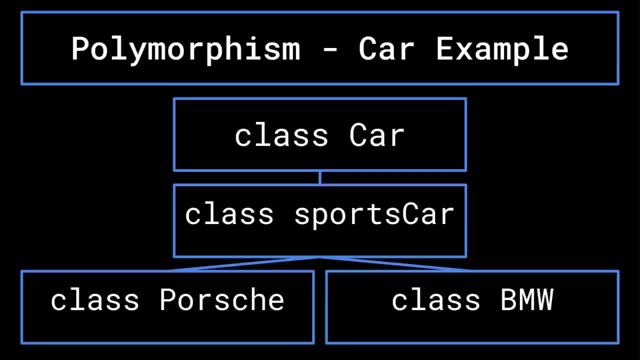 can be extended across a class hierarchy in more layers than just two. You could add more subclasses representing different types of sports cars. For example, if you have a sports car that is called my sports car, my car dot drive will be the same as the car that is called my sports car. This is an example of dynamic polymorphism. 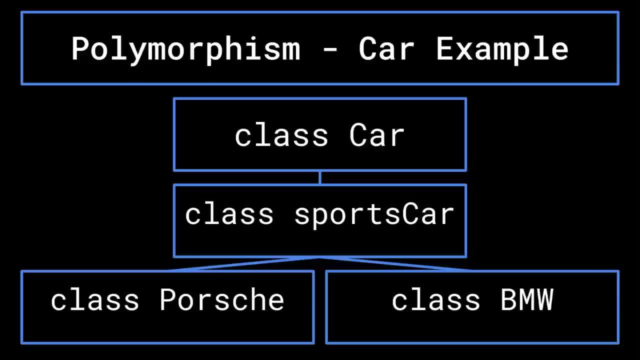 The main benefit of dynamic polymorphism is that it allows you to write methods in the superclass without having to include ifs, and else ifs to account for exactly which subclass is being used when the method is called. The second type of subclass is called dynamic polymorphism. 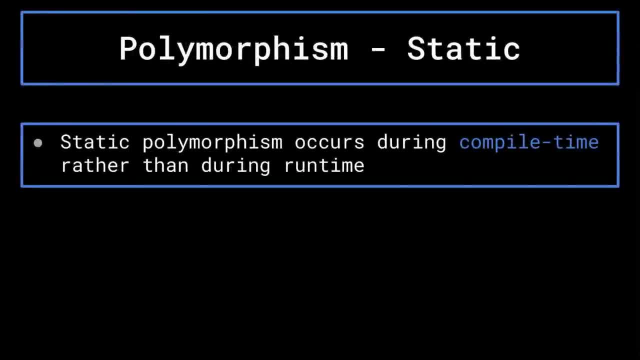 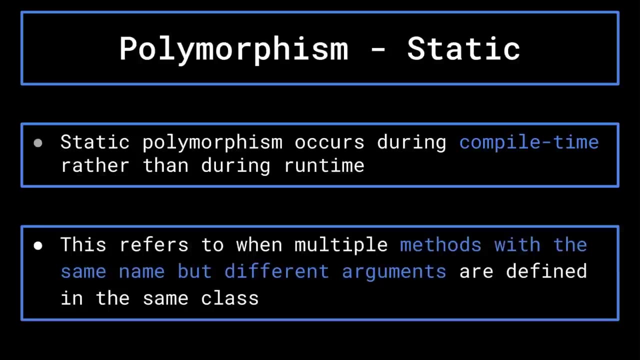 The second type of subclass is called dynamic polymorphism. This is an example of dynamic polymorphism. The third type of polymorphism is static polymorphism. Static polymorphism occurs during compile time rather than run time. This refers to when multiple methods with the same name are defined in the same class. In this case, the methods are differentiated. 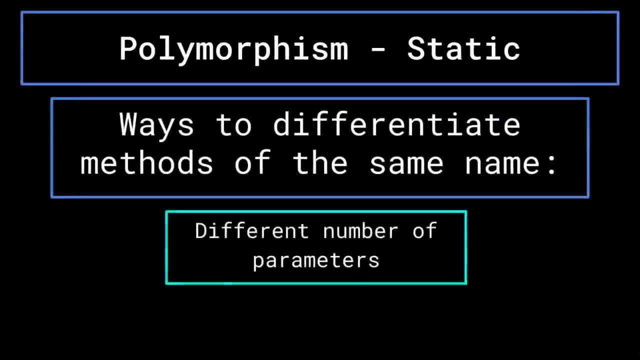 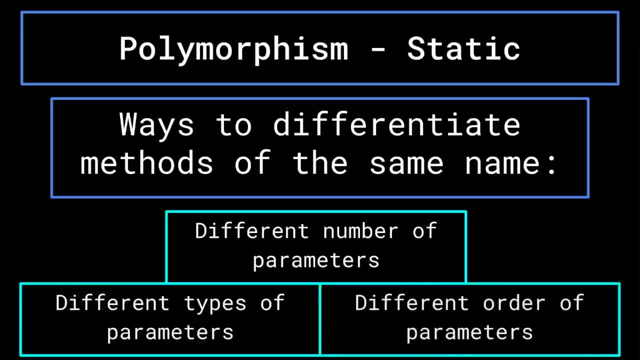 by their arguments. Either they take a different number of parameters, they take parameters of different types, or they take parameters in a different order, depending on which subclass and which subclass is used to determine the same type of polymorphism. The second type of subclass is called method overload. This refers to multiple methods that are different. 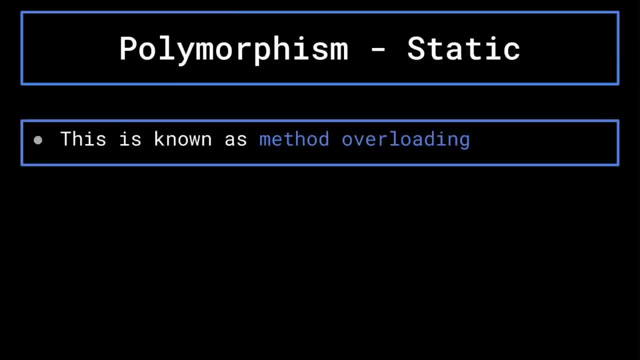 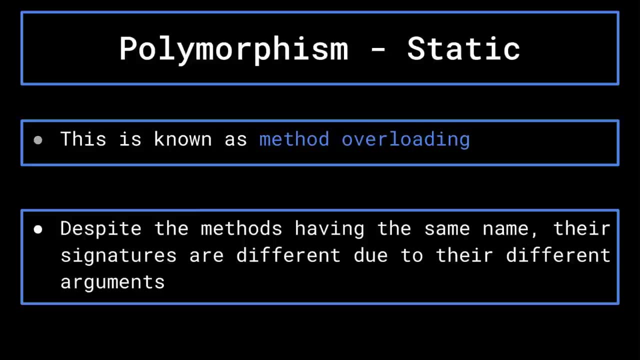 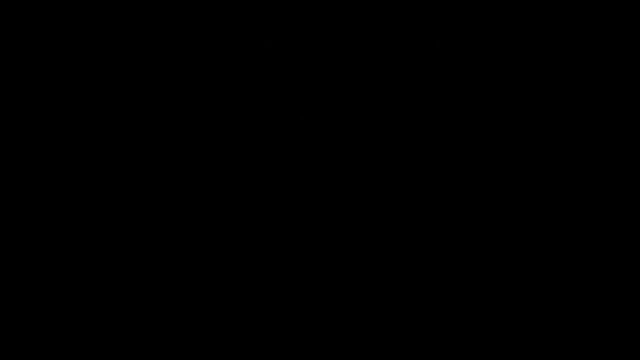 from one another. This is known as method overloading. Despite the names of the methods being the same, they have different method signatures due to their differences in the parameters that they accept. To better understand this, let's go back to the car example. Let's 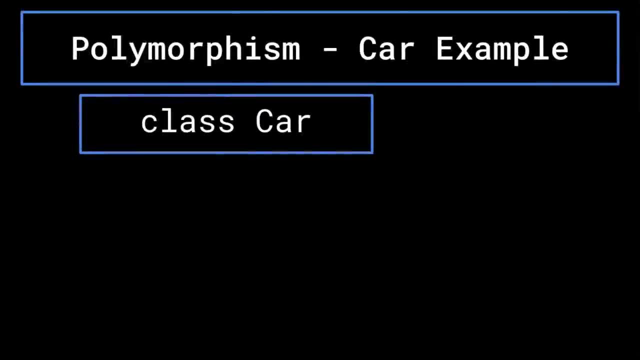 say that you are working within the car class. In this class, you are looking to create three different driving methods. The first driving methods are called drive methods and the drive methods argument accepts one integer and one string as parameters, say speed and destination. For clarity, we will refer to this one as drive method one. However, keep 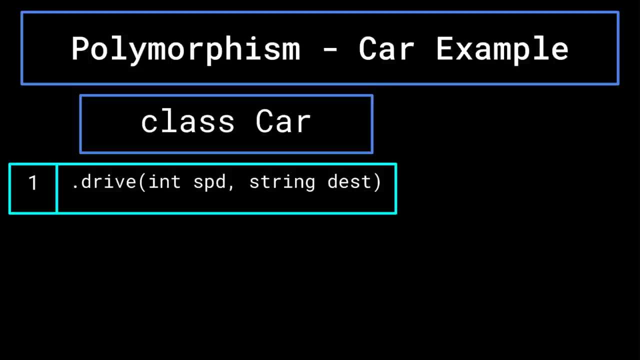 in mind that its method name is just drive. For drive method two, we will set its argument to accept two integers, for instance distance and speed. Finally, in drive method three, we will have it accept a string first for destination and then an integer for speed. 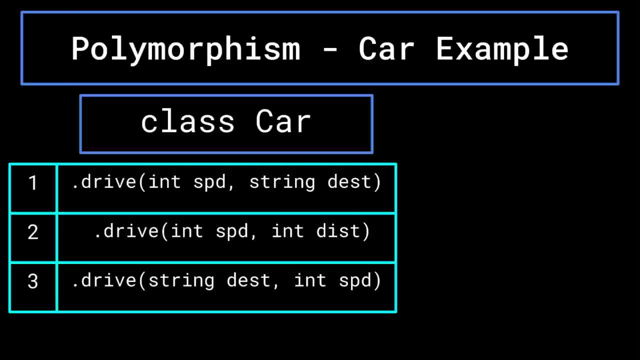 This differs from drive method one, in that drive method one's parameters are in reverse order compared to drive method threes. In each of these three example methods, the method signature is different, despite the methods having the same name, Therefore the computer. 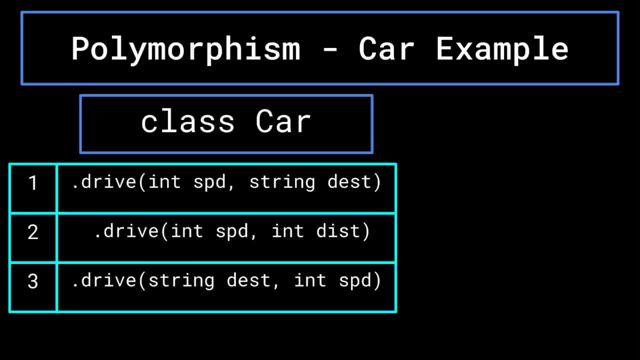 is able to tell the methods apart when the program is being compiled. Okay, For example, were I to call my car dot drive 45, work drive method one would be called, as the argument given indicates that this is the method I would like to call. Furthermore, 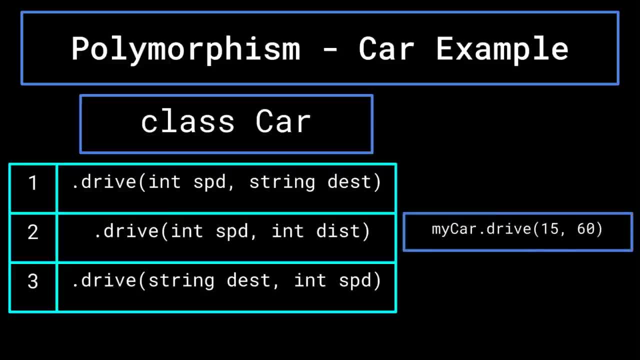 my car dot drive 1560 would call drive method two and my call dot drive school 30 would call drive method three. When implementing method overloading, the different methods tend to have separate but similar effects, Despite drive method one and drive method three taking the same. 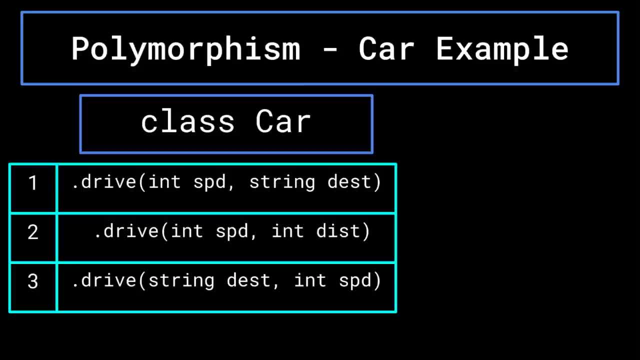 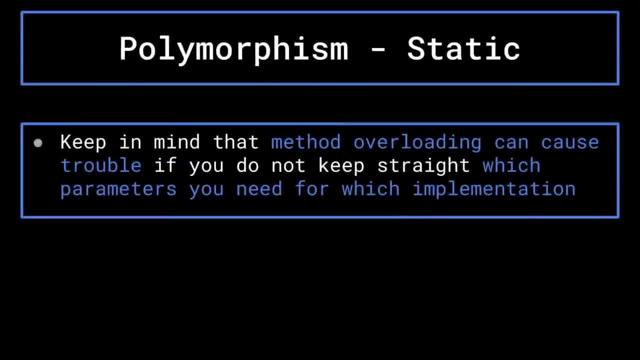 parameters, it is likely that their implementation will be different and thus would achieve separate effects. Otherwise, there would be no reason to have both methods. Keep in mind that method overloading can cause trouble if you do not keep straight which of the methods. 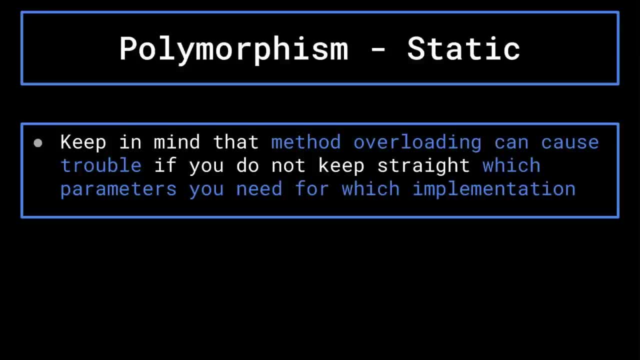 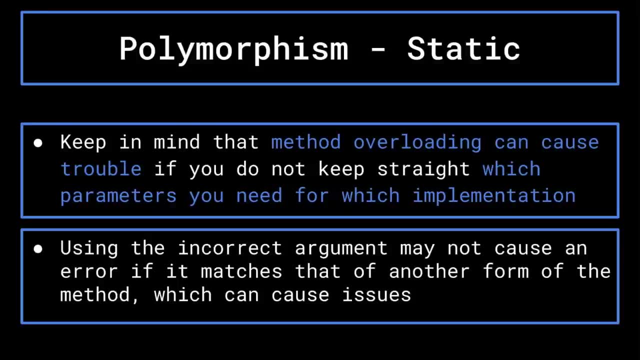 implementations you would like to execute and what form of the argument is required to do so. Normally, if you call a method with too many parameters or parameters of the incorrect type, then the program will throw an error and you will be able to fix the issue. However, if you mistake the method's, 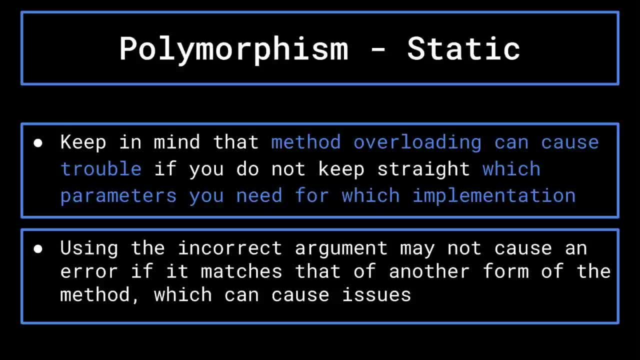 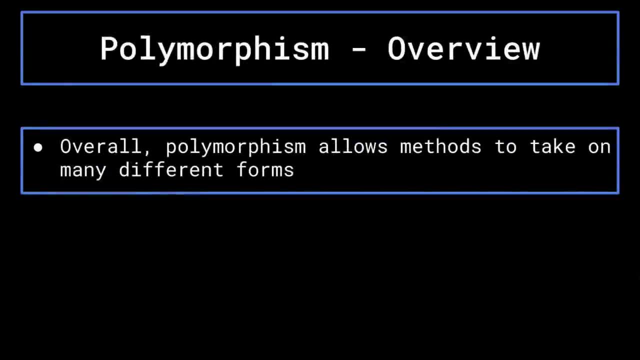 argument in such a way that one of the other methods with the same name is called instead, then you may not even be aware that you made a mistake. Overall, polymorphism simply allows methods to take on many different forms. It can be very useful in that it allows methods. 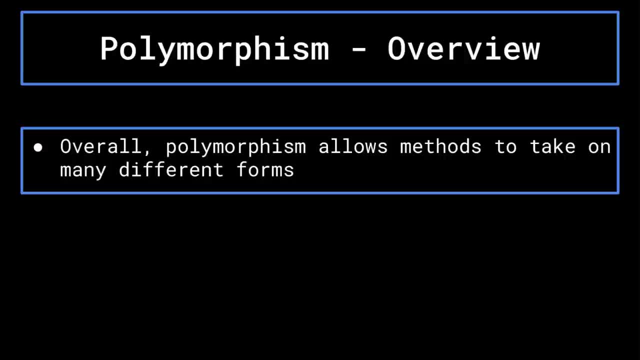 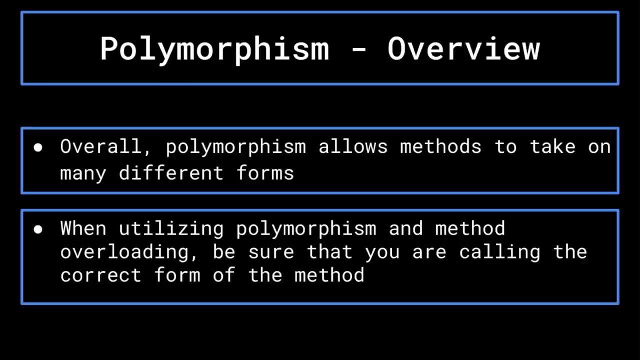 of the same name to exist both in the same class and in different classes. However, you must be careful to ensure that you are calling the correct form of the method that you want so your program can function as intended. That does it for polymorphism and with the 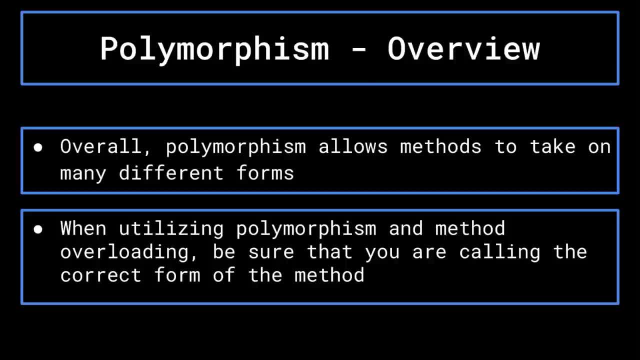 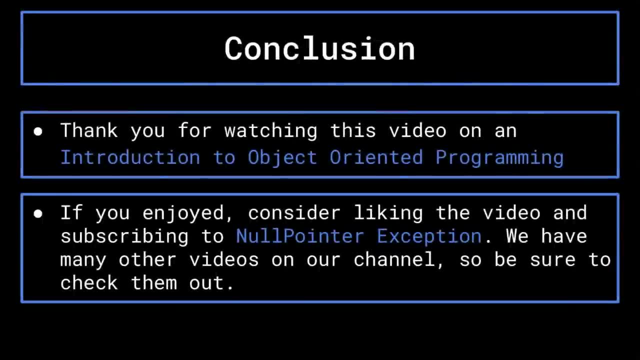 end of polymorphism- the final of the four main principles- comes the end of this video on an introduction to object-oriented programming. If you enjoyed, consider liking and subscribing to the channel, Thank you. Thanks for watching. 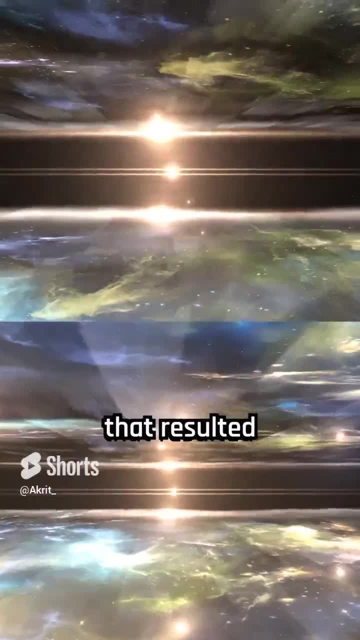 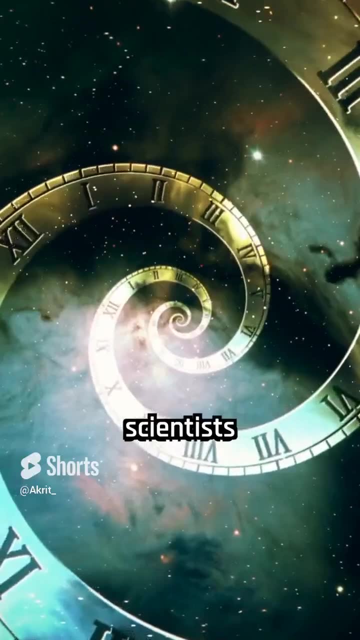 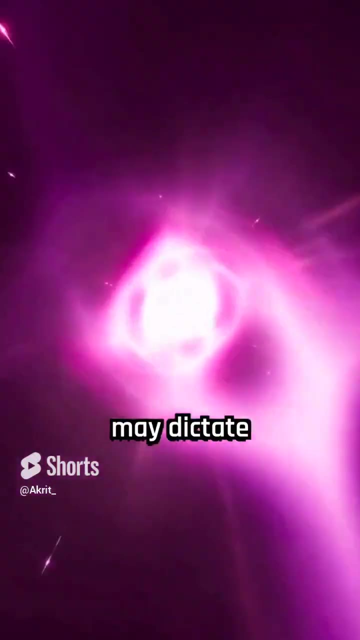 Physicists have created a simple Big Bang simulation that resulted in the formation of two universes, with one universe moving forward and the other moving backward. For over a century, scientists have sought to explain the direction of time, and one explanation suggests that gravity, rather than thermodynamics, may dictate the flow of time in our universe. 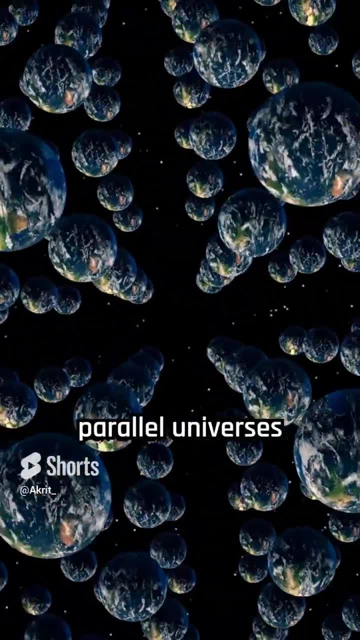 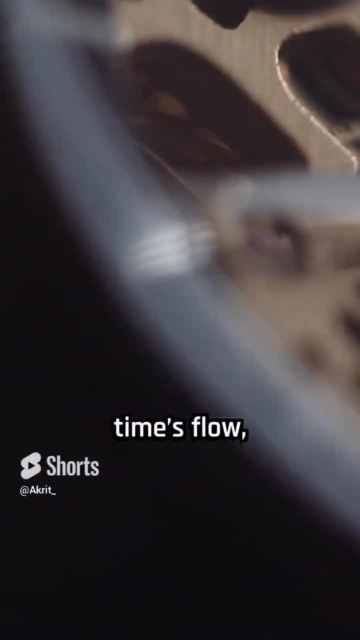 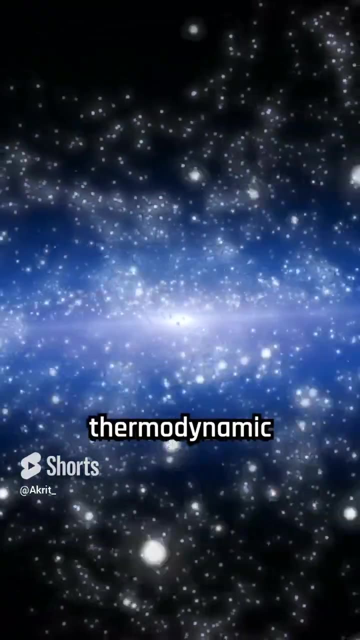 According to this theory, the Big Bang could have generated parallel universes where time progresses in opposite directions, While the fundamental laws of physics remain consistent, regardless of time's flow. our universe follows a single arrow of time. This phenomenon is attributed to entropy, which measures the disorder within a thermodynamic 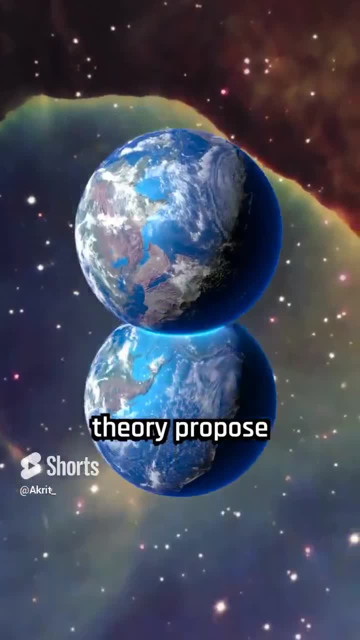 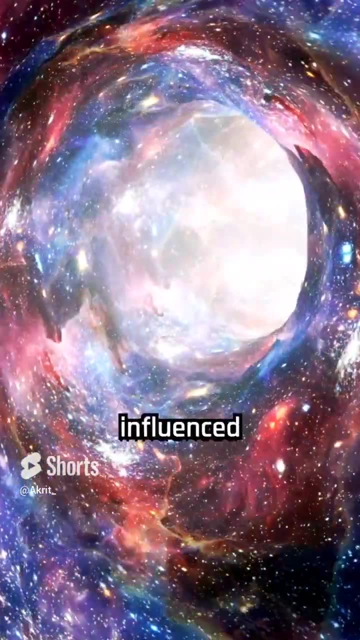 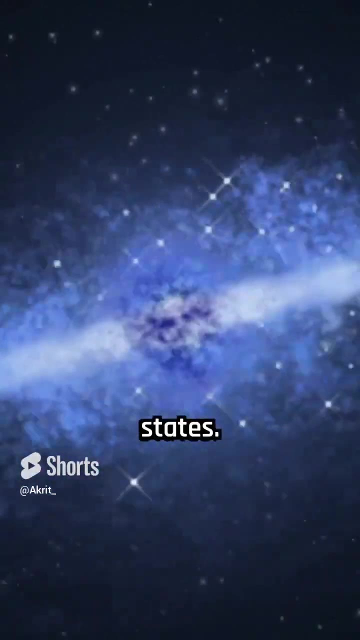 system. However, proponents of the parallel universe theory propose that gravity is responsible for the unidirectional flow of time. Through computer simulations of particle interactions influenced by Newtonian gravity, researchers observed the particles coalescing into densely packed low-complexity states. These states then expand, creating two different.